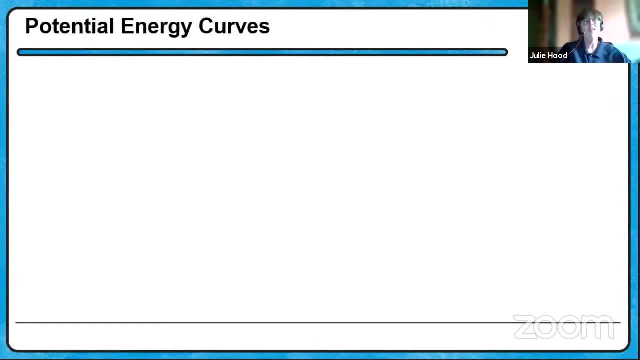 So today we're going to study potential energy curves, We're going to review that topic, We're going to go ahead and we're going to look at graphs of potential energy functions and their associated forces. We're going to be applying the law of conservation of energy a lot so we can determine how particles behave in this mechanical system. 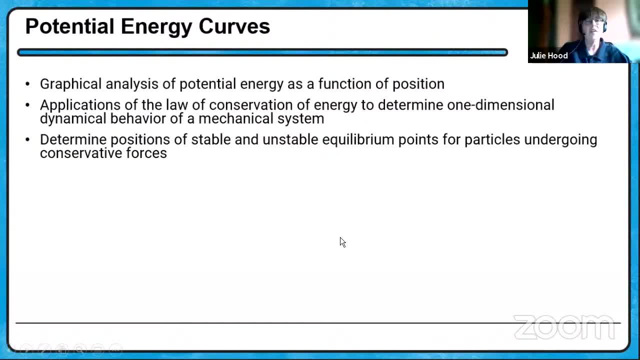 And we're definitely going to look at stable and unstable equilibrium points- and I'll show you how to do that- And because we're dealing with conservative forces, we're going to be able to determine the force from a potential energy function And by doing so, 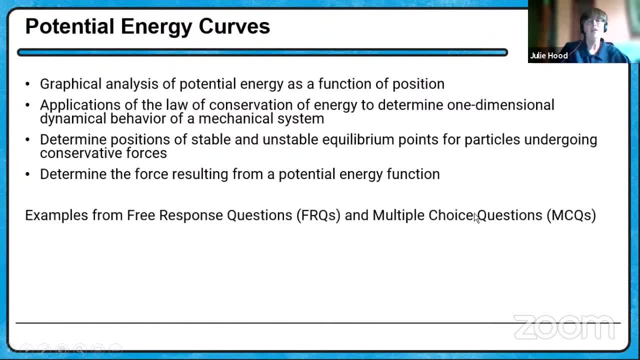 versa, And we'll definitely look at some free response questions and some multiple choice questions from old AP exams so you'll get a good idea of what's expected of you. And you know, in addition to the few I go over today, the free response questions are housed on AP Central Just. 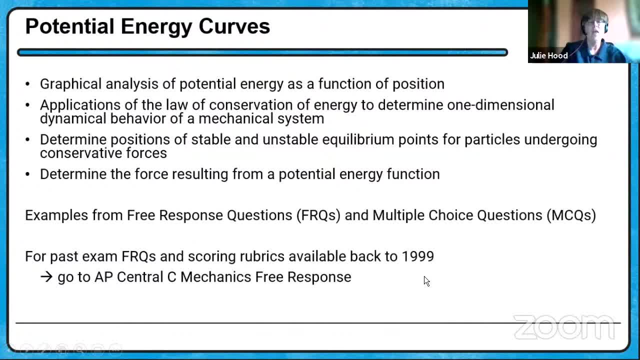 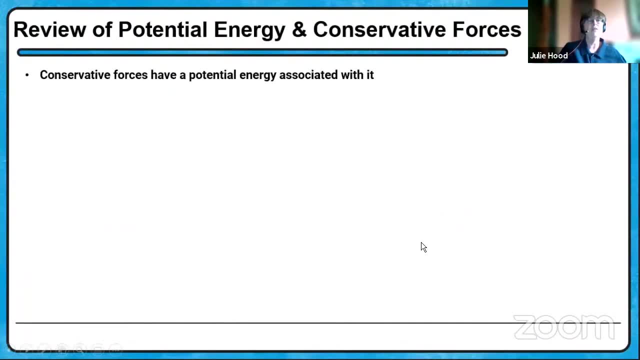 Google AP Central, see mechanics, free response, and you can find free response questions and their scoring rubrics all the way back to 1999.. Practice, practice, practice. So let's review what we're doing today. I mentioned conservative forces earlier and they 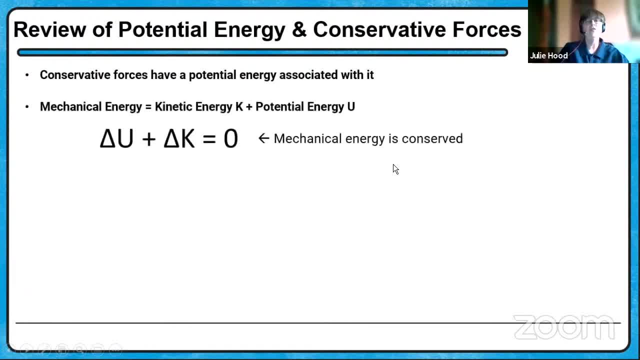 always have a potential energy function associated with them. A conservative force means mechanics and energy are conserved And there's a trade-off between potential and kinetic energy, And the difference in the two is half to equal zero. Mechanical energy is conserved when you have. 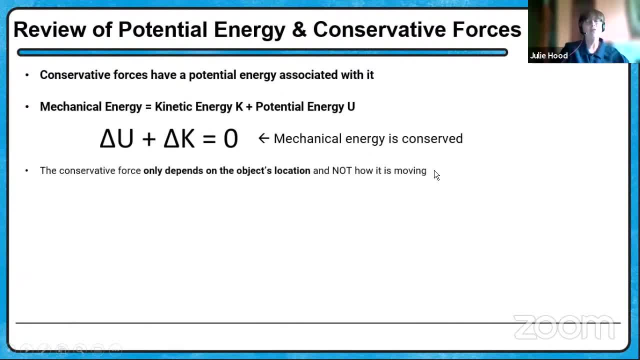 a conservative force, By the way, a conservative force, it only depends on your location, not how the particle is moving. So it's also- I'm sure you remember this in calculus. but work done by a conservative force is path independent. It doesn't matter how. 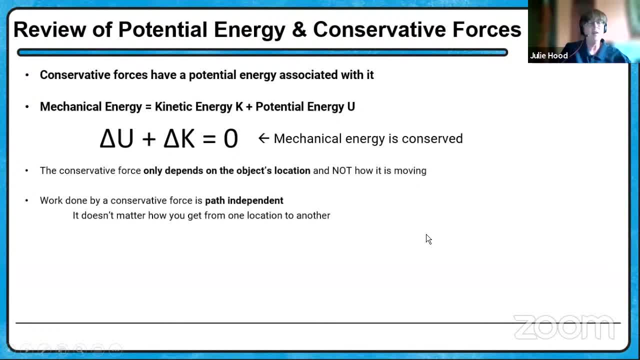 you get there. If you go from point A to point B in a straight line, well, good for you. You've done a certain amount of work. But if you go in some circuitous, crazy, loop-de-loop way of going from A to B, you'll still do the same amount of work. Now here's some forces that are not. 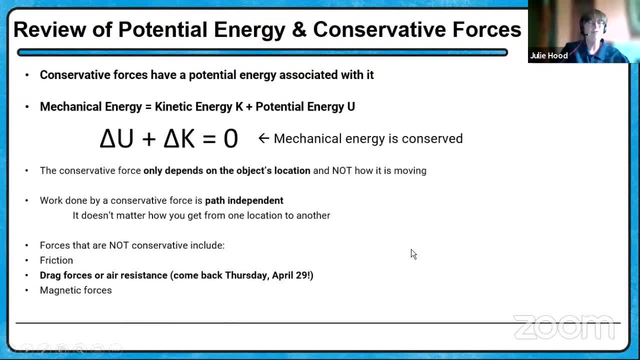 conservative Friction, Magnetic forces And hey, you know how they always say: neglect- air resistance. Well, if you have to take into account drag forces and air resistance, then you don't have conservative forces and you can't assume mechanical energy is conserved. I suggest you come back next Thursday. 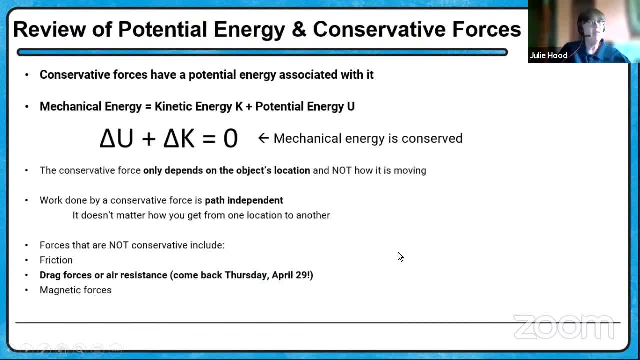 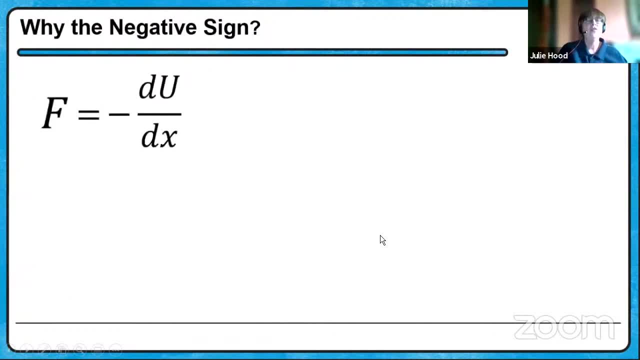 April 29th and I'm going to be talking about air resistance and resistive forces all day long, Thank you. So, first of all, we're going to use this equation a lot, a lot, a lot. And you know why the negative sign? Seriously, why the negative sign? Well, I'll tell you why: Because 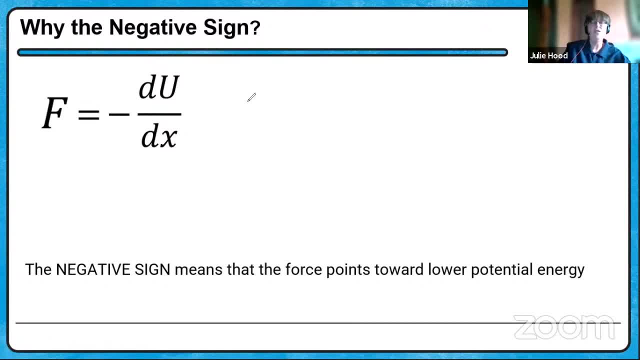 the force always points towards lower potential energy. Let's say: you've got a hill and you've got a rock, you know, and there's this little pebble wedging there. The rock wants to roll down the hill to a lower potential energy. And if you look at this right, I'm going to go up the 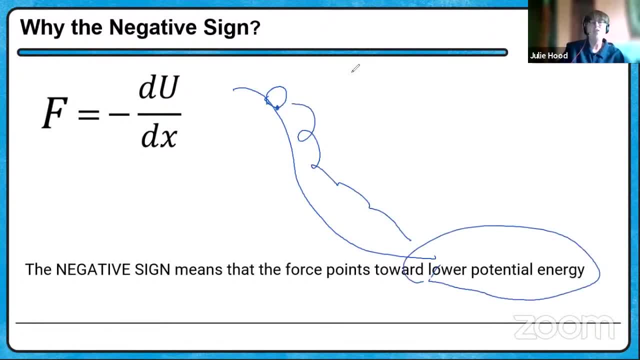 potential energy. So the force points down the hill. Now, if you want more information about this, then I suggest you check out some AP Daily videos. Mr Frensley did a whole series of videos in unit three, topic two, in particular, and they are great, And he actually derives this equation for 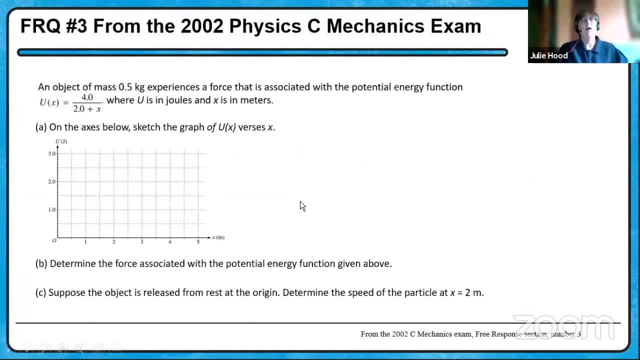 you. So let's practice. Here's a free response question from the 2002 exam And we're given a potential energy function, a mass of an object, And the first thing they want you to do is graph the function and then determine the force associated with it. And then they want you to 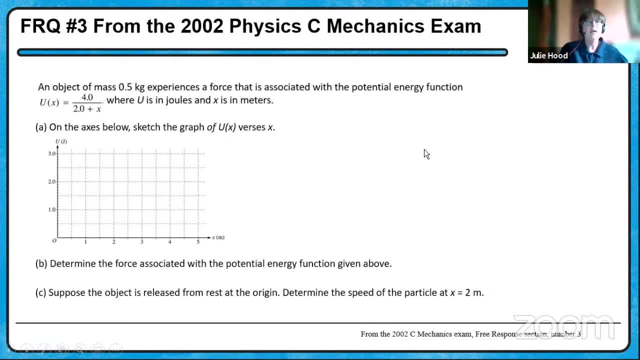 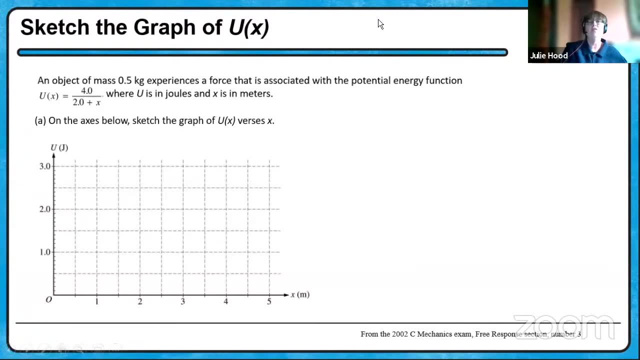 calculate the force associated with this potential energy function. And finally, we're going to release the object from rest when it's at the origin and figure out how much speed it would be when it gets to x equals two meters. So let's try that. First thing we have going on is sketching. 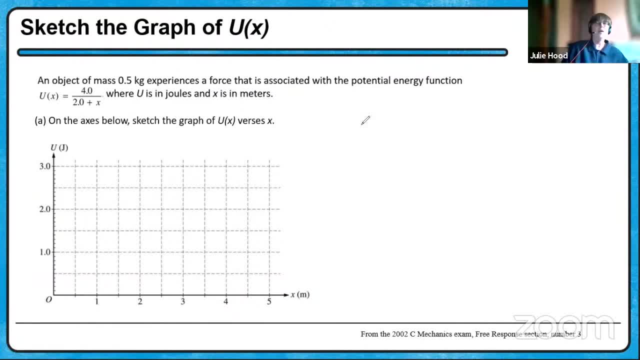 the function. You can do that. I mean, if you have a graphing calculator, by all means use it and then sketch in the function. Or if all else fails, hey, just you know, write your function here. That's a four, by the way, Two plus x, Okay Well. 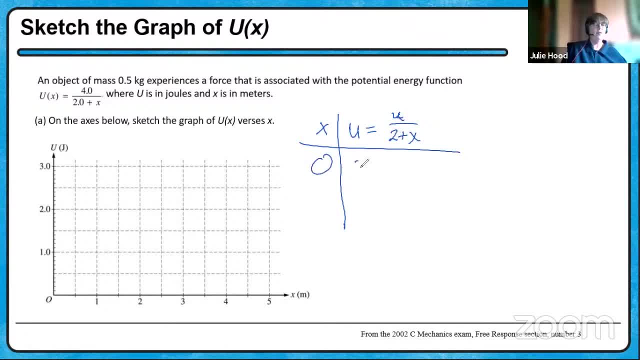 what happens when x is zero? Well, four over two is two. So guess what? That point is part of your curve. What happens when x is oh, I don't know how- about a two in the denominator That makes this four over four, Oh one. So when we're over here, at x equals two, our potential energy has one. 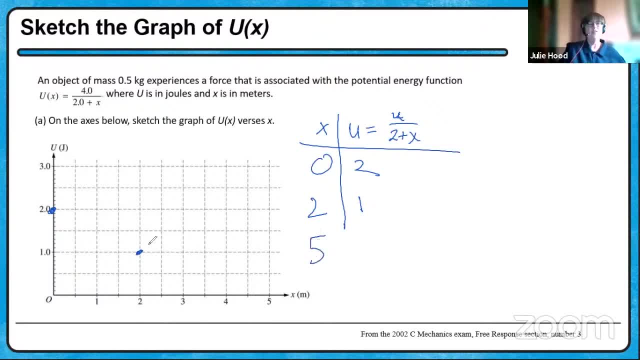 Hey, why not When x is five? you know, when x is five, let's see. I see that the curve's probably going down. But when I put five in, okay, the potential energy is four sevenths joules, You know. 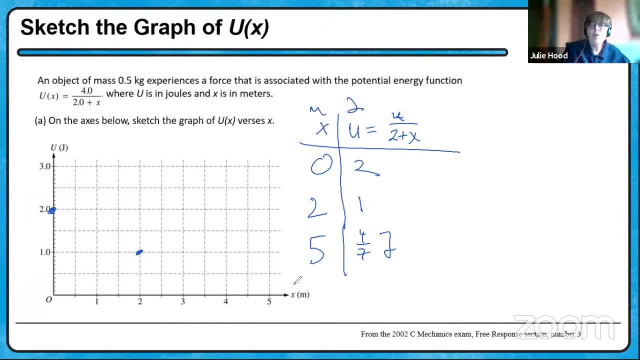 these are meters, These are joules, And four sevenths is a little more than a half. Here's a half right here. So you want to do a nice smooth sketch, Probably nicer than what I have, But hey, that's not bad. 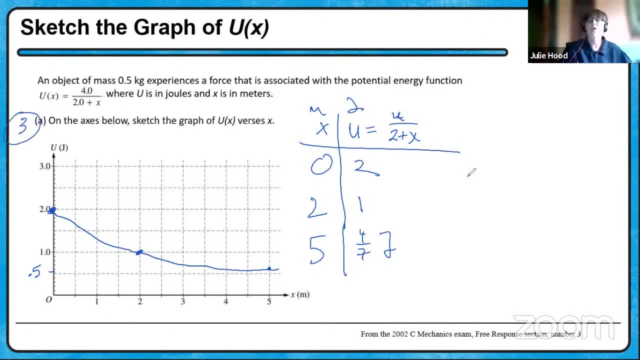 This part of the problem was worth three points. Remember all your free response problems. there will be three of them and they will each be worth the same 15-point value. And there's three of them And you have 45 points And you have 45 minutes, coincidentally. 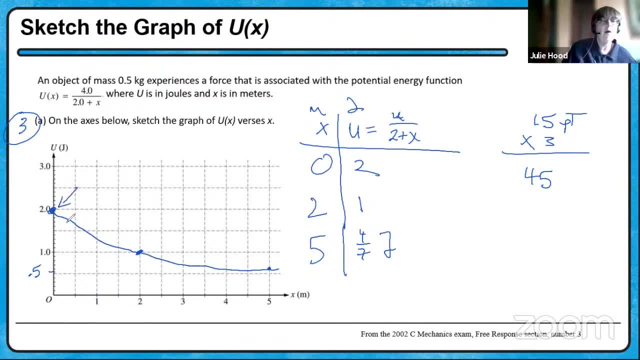 This three points. you got one point by making sure that the u-intercept was at two. So hey, I've already earned a point. They also wanted to see the curve go through the point to one. All right, And you know. 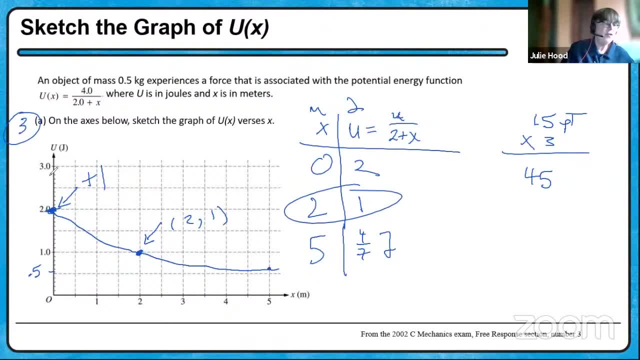 there it is, And you know you had to have your curve going be concave up, monotonically approaching some value. when x approaches finity, It basically approaches, you know, a very small number, But out here we're only going out to five. 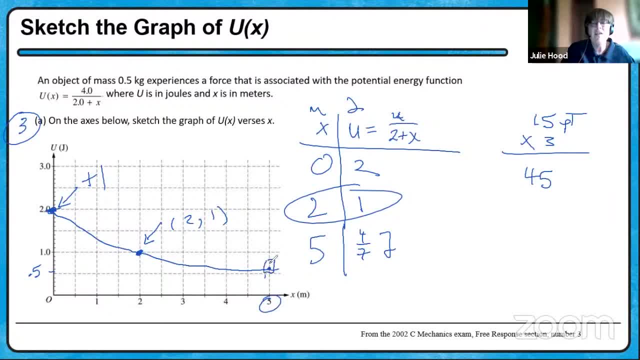 And as long as your curve lied somewhere between here, they actually said between 0.5 and 0.75.. They were pretty generous And I say we met it and we got our third point out of the deal. So hip, hip, hooray. Now let's see what we've got going on in our next slide. Oh, now we need to. 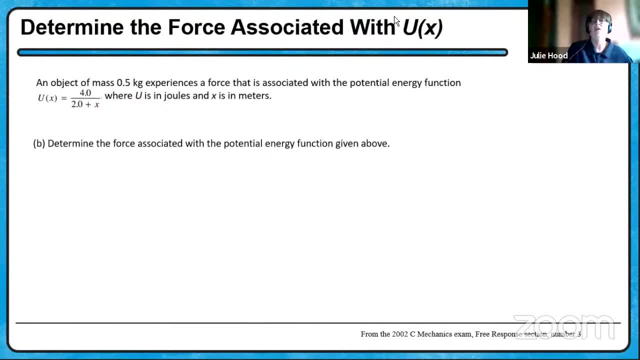 determine the force. Well, remember that function I wrote up a while ago: The force is the derivative of the potential energy curve. It's literally the slope of the potential energy curve, but negative because the force always points to go to a lower potential. So we have to write down. 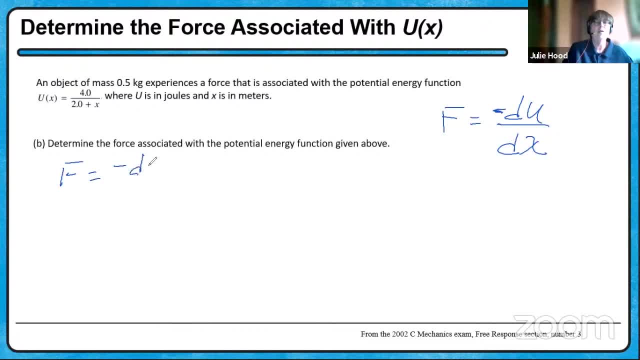 our equation. I know I wrote it up on the side here, but let's just make it easy on the people grading your AP test. All right, so I've got to take the displacement derivative of the potential force. All right, so this derivative will give me a negative. 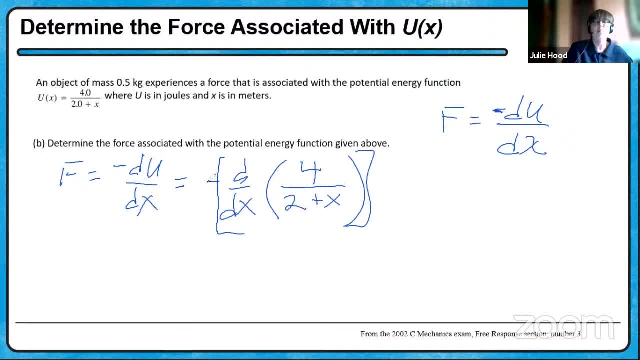 for two plus X in the denominator squared, but don't forget about the negative sign upfront. So we're gonna end up with four over two plus X squared. Yay, I know how to take a derivative. That will actually be worth one of the four points. 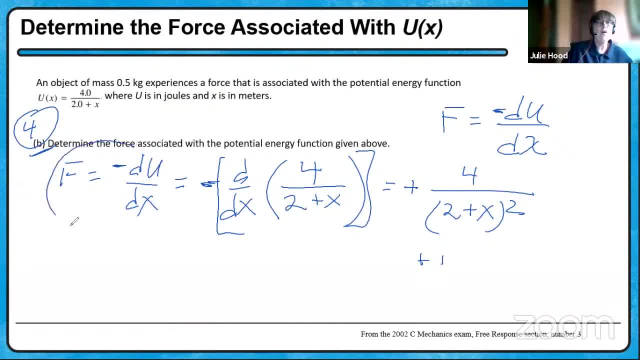 This part was worth four points. They gave you one point just for writing the equation down. They gave you a second point for remembering that there's a negative sign. We got a point: We're getting the right derivative. And we got our fourth point by using: 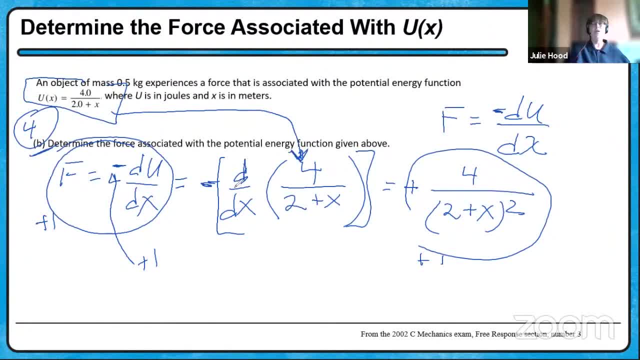 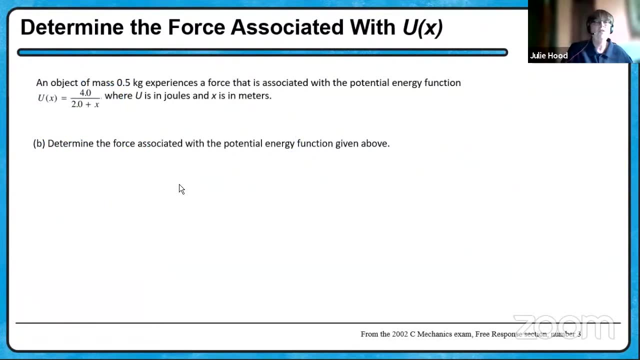 the potential energy curve, knowing that we had to take the derivative of the potential energy. So good for us. We got all four points In fact. wow, we've already done seven out of the 15 points. I gotta tell you when you're doing these problems. 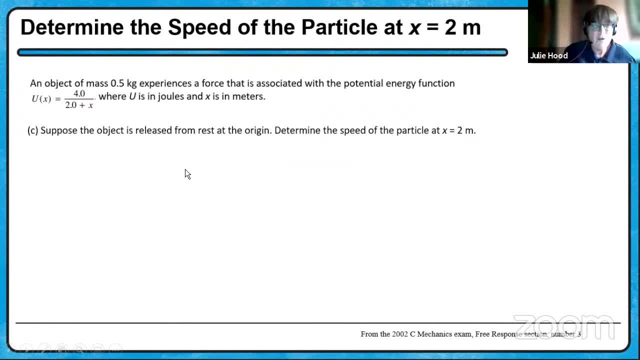 you know, read through the whole test, see which problem looks most doable for you and don't pass up the easy points. Go back and if you still don't know how to do a few crazy things, then do the easy stuff, all right. 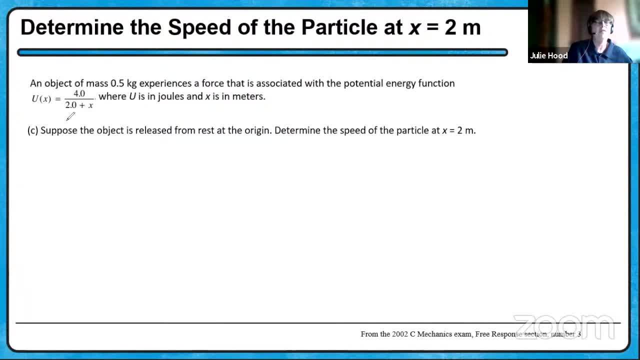 Like graph and free body diagrams and take a derivative of a simple function, things like that. Now, this third part was worth three points, and here's what we're saying. Here's our function. The object, suppose it's released at rest at the origin. 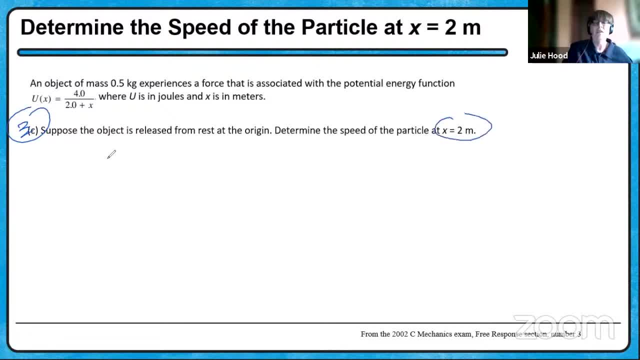 Determine the speed of the particle when we're out here at, x equals two. Well, look, energy's conserved, And if that's all you wrote down, you would get a point. Now you don't necessarily have to use the words. 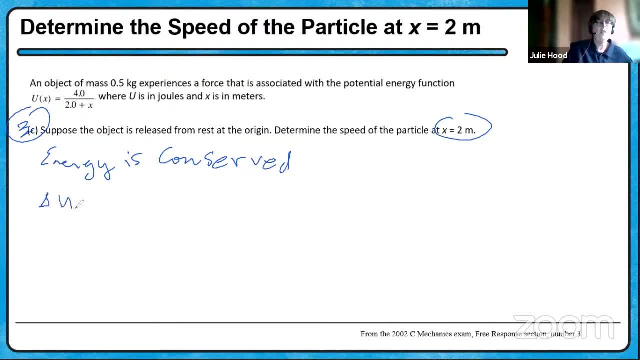 You could express that the way I did in one of my opening slides, that the change in potential plus the change in kinetic has to amount to zero. Mechanical energy is conserved because you've got a conservative force. So at the origin they're telling me that. well, 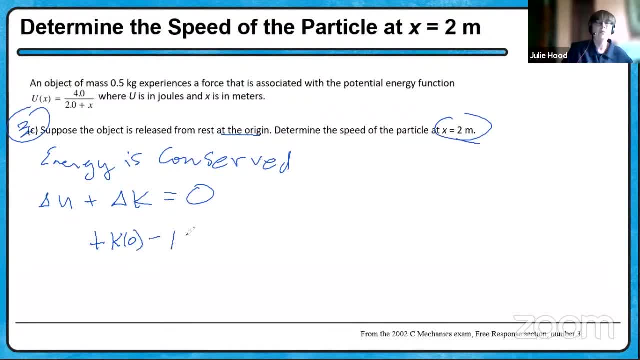 let's just plug it all in. We're going to go out to two And you at zero and you at two. So at the origin they're telling me that the objects that rest hey kinetic energy. if something's at rest, it has no kinetic energy. so, um well, let's see what is. 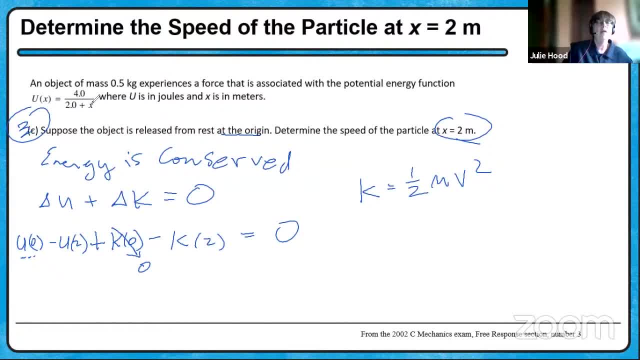 u at the origin. we plug in a zero, we have four over two, oh, two joules, and what is the potential energy out at two meters? well, we put a two in the denominator there. two plus two is four, four over four is one and we have the zero and we have. well, let's just move k2 over here and k2 is one half m. 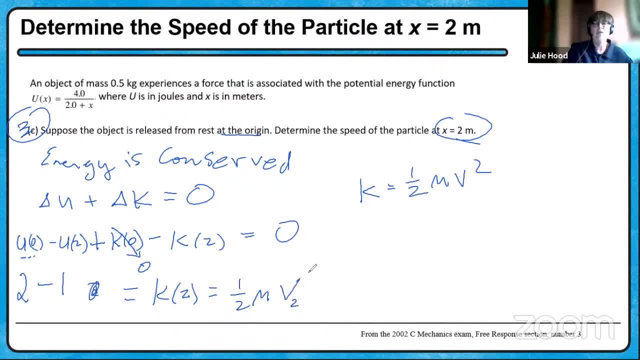 v at position two meters squared. uh, two minus one is one. so now we're down to this right here. let's solve for v. well, v2 squared is going to be two times your potential energy out at two meters squared. so we have two minus one is one. 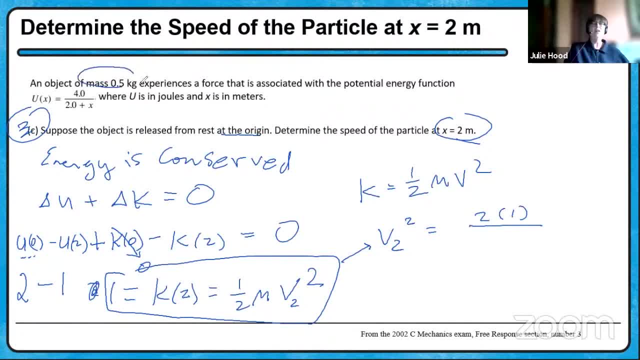 energy one joule divided by your mass- hello, there's your mass one half. that means what's two divided by a half, it's four, and this is velocity squared. so when you take the square root, you find out that your velocity is, you know, plus or minus two meters per second squared. but 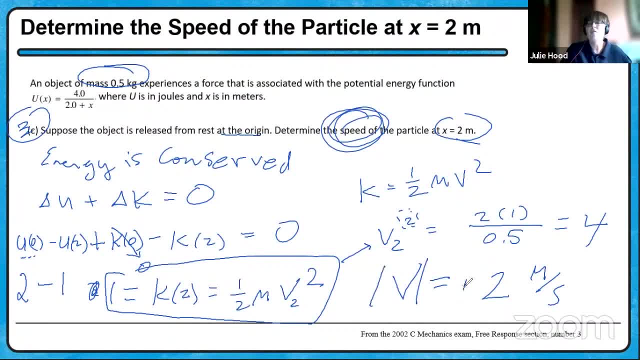 we're looking for the speed, which is the absolute value. and there you have it. this was worth three points: one for this one or the other statement of energy conservation. two, uh. the second point for actually evaluating um that statement at these positions: origin and two meters. and finally the third point. 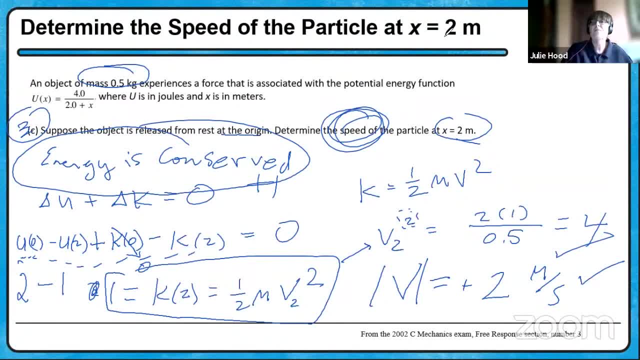 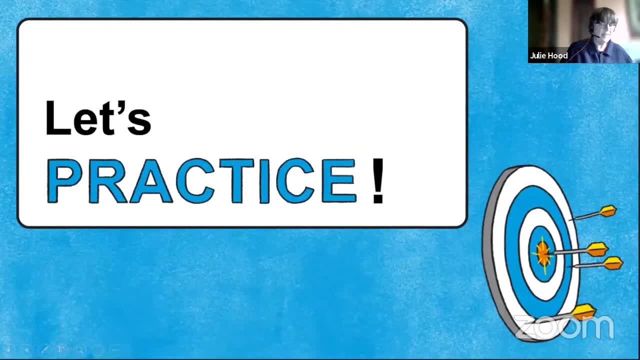 for getting uh the calculation correct. all right. why don't we see what's going on with um part d? well, it's not there. i will let you look it up. it has more to do with selecting lab equipment and outlining a procedure to uh determine experimentally the validity of that calculation. 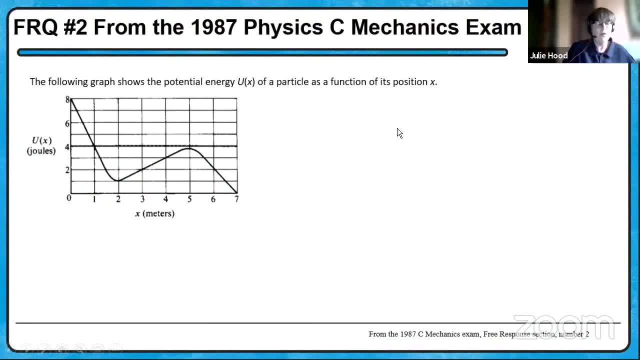 and part c, but um, i'm focusing more on potential energy curves today. now here is another free response problem. this one is from the 1987 exam, and what they give you is not the answer to the question, but rather the graphical uh depiction of that function. so here's the potential energy. 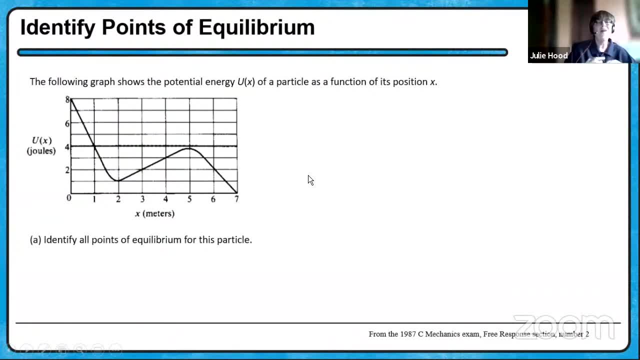 curve and the first thing they want you to do is find the points of equilibrium. now, in calculus- you should have heard this term- points of equilibrium are when the uh derivative is zero, so the derivatives, since the derivative of the potential function with respect to action is zero. so the derivative of the potential function is zero, so the derivative of the potential. 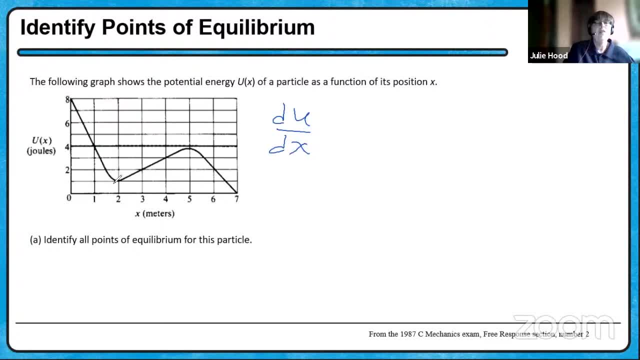 function is zero, so the derivative of the potential function is zero. the derivative of the potential function is zero. so a next step in the the you know the helix is the slope of this curve. the- uh, you're gonna sketch in tangent lines. oh, all the same, all. 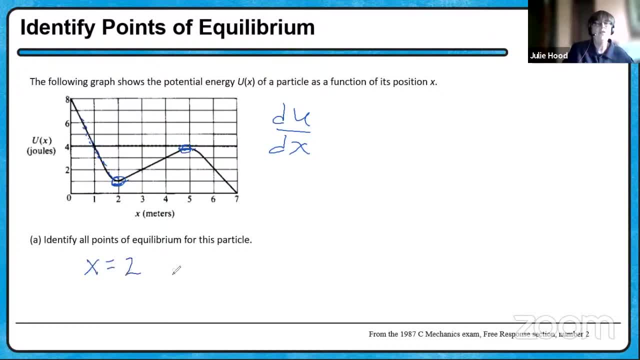 the same. oh, tangent line, tangent line, horizontal slope is zero. yeah, where the turning points are points, That's it. Now, they gave you three points, one for each of these and a third one if there weren't any extraneous points, if you didn't list any other points, And I don't know. 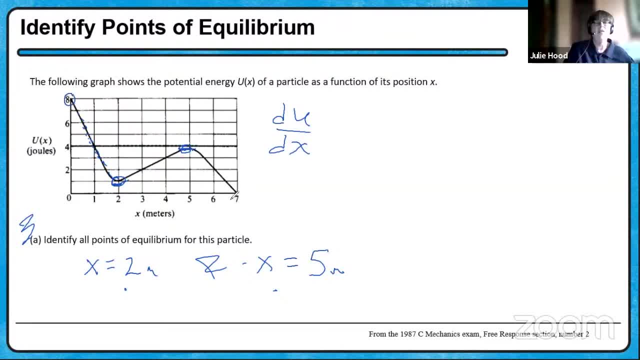 what you might have listed. Maybe someone thought at the origin or out, at seven there was an equilibrium point, But we don't know what the function's doing beyond those positions, So don't don't over guess. Now, the next part of this question wanted us to find: 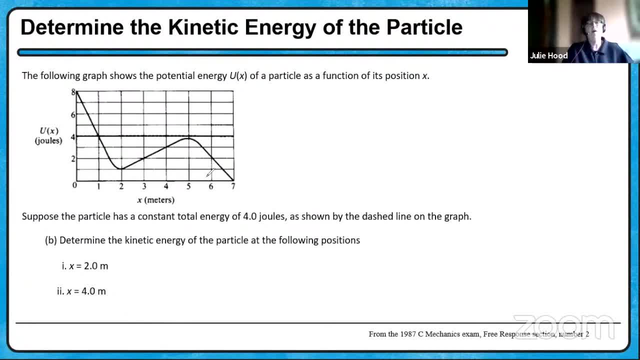 kinetic energy of particles when they were at these different positions, Okay, at two and at four. Now they tell us that the particle has a constant total energy of four joules. And if I find, if they give it to me, great, But if I find a constant total energy of four joules, 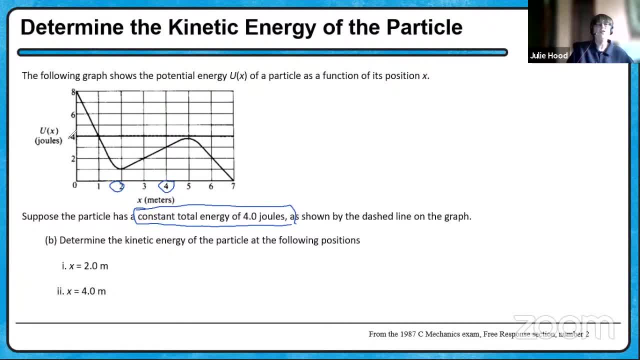 I go ahead and I make a horizontal line right there, And actually they did. They showed it with a dash. There's apparently a dashed line there. There's your horizontal line, And what that means is the particle can't exist up here. And what up here means is the particle can't get. 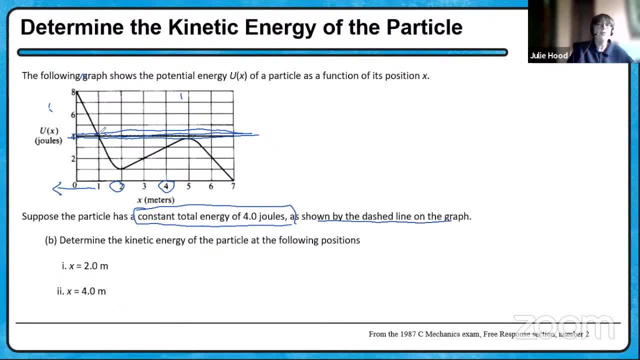 beyond. go to the left of x equals one, And well, it looks like it can certainly get to the right, at least all the way to seven metres, because we have enough energy to do so. At two metres we're below that horizontal line. In fact. we only need one, one joule of energy there. 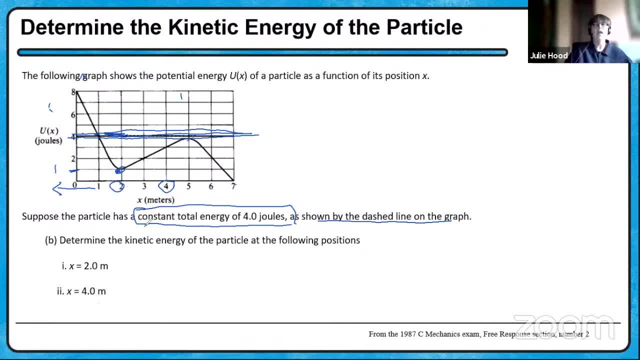 So it's moving fast, it's got kinetic energy, And so hey, um, actually, what they ask is determine. Oh, we're determining, Oh, we're determining, determining, determining kinetic energy. Of course we are. So the total energy is the sum of potential and kinetic. 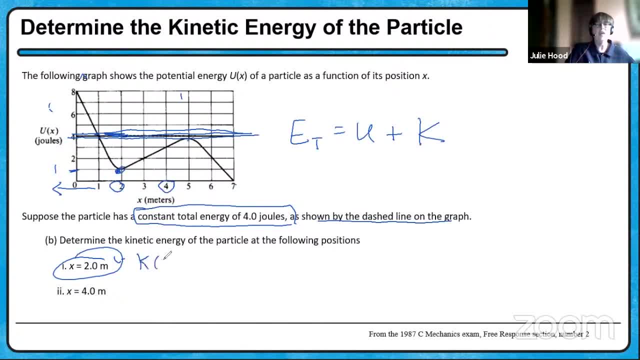 Okay, So at x equals two, the kinetic energy is going to be the total energy minus u at two. Well, what is u at two Right here? Read it off the graph: It's one joule. The total energy is four. That's a given, And the potential energy at two is one joule. So the kinetic energy right here, 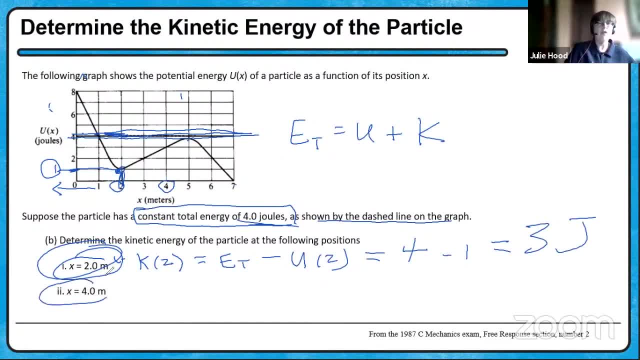 is three joules. Do the same for x equals four. Okay, Kinetic energy at x equals four is going to be your total energy, which is four joules minus well, what's u at four? Read it off the graph. It looks like three to me. So we have one joule. 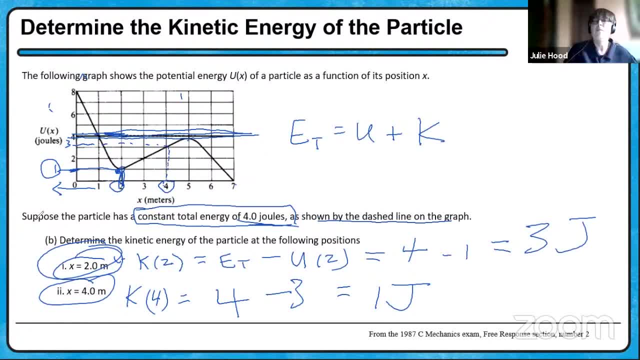 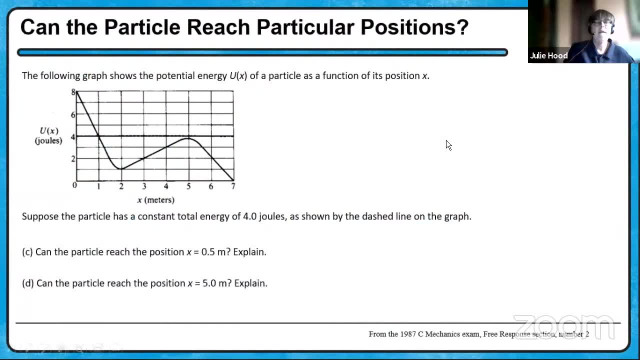 So we have one joule of kinetic energy at x equals four. Okay, I like that Now. now we get in. I got ahead of myself, but we still have total energy of four. But can the particle reach 0.5 meters? Here's 0.5 meters. Can the particle get there? Well, let's see how much. energy it can get, Okay. So we have a total energy of four. So we have a total energy of four. And we have a total energy of four. So we have a total energy of four. So we have a total energy of four. 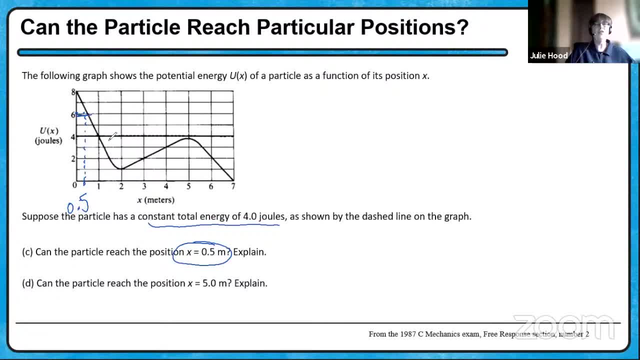 Oh, it would need six joules of energy And it only has at most four. So no, it can't get there, There's not enough energy. Don't just say no, Say why, Explain, You won't get a point, for just. 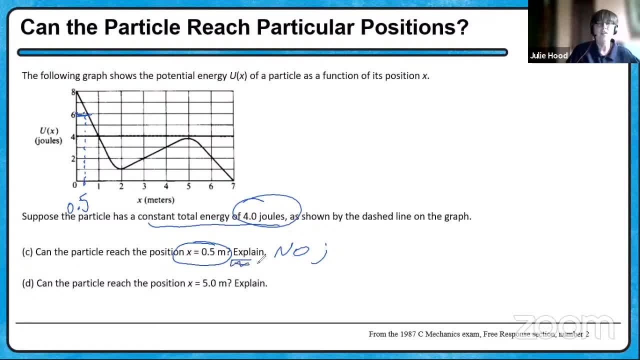 you know checking a box or saying yes or no, Not when they say explain. Well, explain, There's not enough energy. Go ahead and use words. That's good enough. Now can the particle get out here to five? Well, yeah, it has enough energy. Remember. 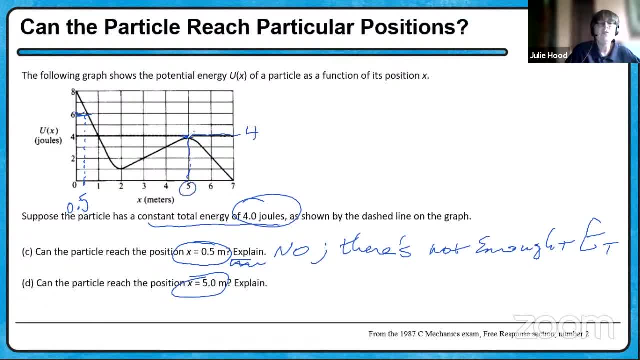 it has four joules of energy And at x equals five. they're slightly under four joules tied up in potential energy. So there's a little bit left for kinetic. It can get there. Yes, Sufficient energy, Boom, boom. I would understand that abbreviation and give you the answer. 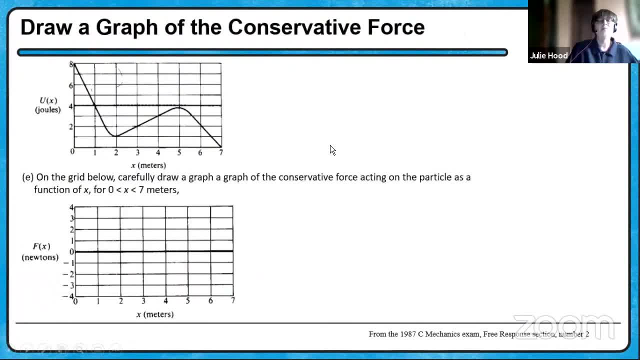 I would give you full credit. All right, Now here's the fun part. What if we're back to having the curve and we're asked to sketch or draw carefully, carefully draw, a graph of the conservative force? Oh yeah, This equation- This, by the way, is not on your equation sheet. 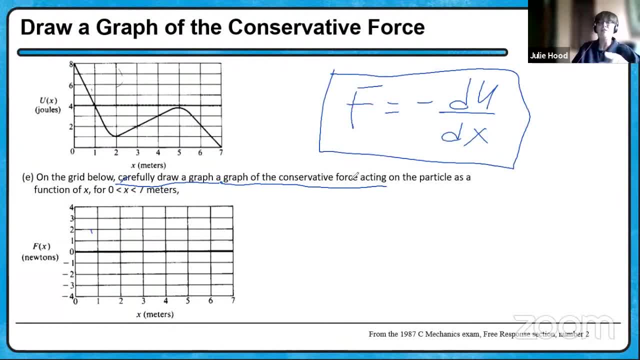 This equation only works when it's a conservative force. It's worth remembering This is a slope, So these are nice little straight line bits. Sure, There's transitions: at x equals two and at x equals five. Something's going on there. Let's. 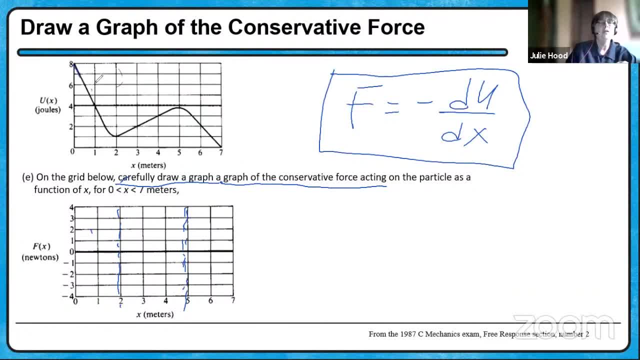 figure out what Well the slope in this region is. let's see rise over run Eight, seven units minus over two units. So the slope is minus three and a half. But remember the force is negative slope. So we'd. 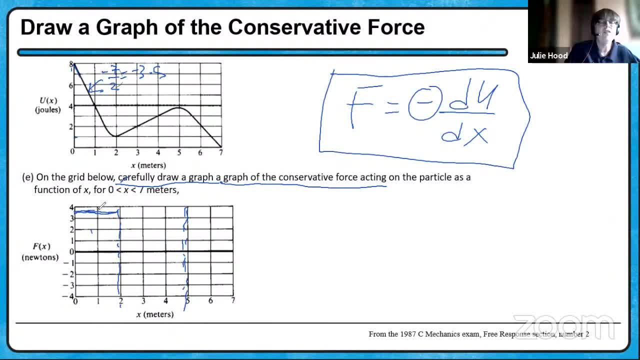 go up here to three and a half and we'd literally sketch the force with a nice horizontal line. Likewise, let's find the slope here. Rise over run. Rise is about three units, Run is the same. It looks to me like the slope is a positive one. So again, 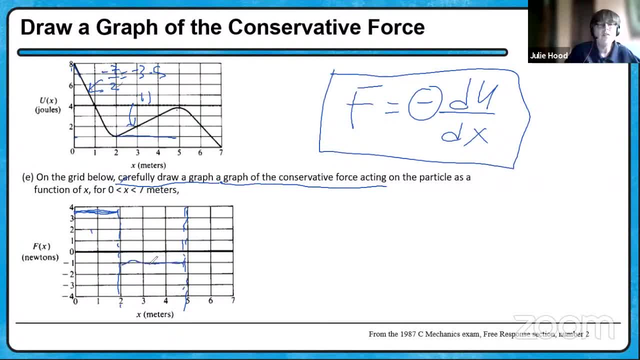 force is negative. So negative one. There it is. That's supposed to be a nice horizontal line. And what's your slope here? Well, let's see It's negative and it's rise over, run four over two, about minus two. So we got to go up there to two. So this is our and do a little. 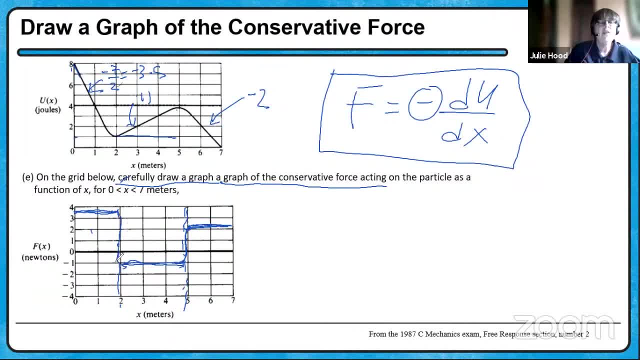 smooth transition, like you would in your calculus class, And there's your force function, That's it. That's the force And that's its associated conservative or potential energy. Yeah, Good stuff, All right, And that was the entirety of that problem. We have one more I want to work with you on today. 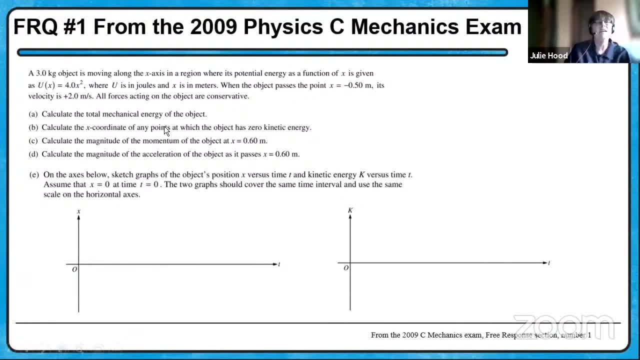 And this one is from the 2009 exam. It was number one And, oh my, there's a lot going on, but don't worry, I'll break it down. They give you. they give you a nice elegant data loop of mass and they give you the potential energy, And so you know what the 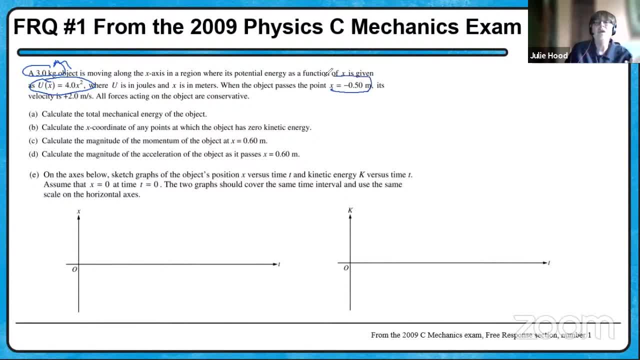 total energy is, They tell you when it's located at a certain position, it has a certain velocity. That's going to be some really good information. We're going to need that. In fact, in the very first part we're going to calculate the total mechanical energy and then we're going to find 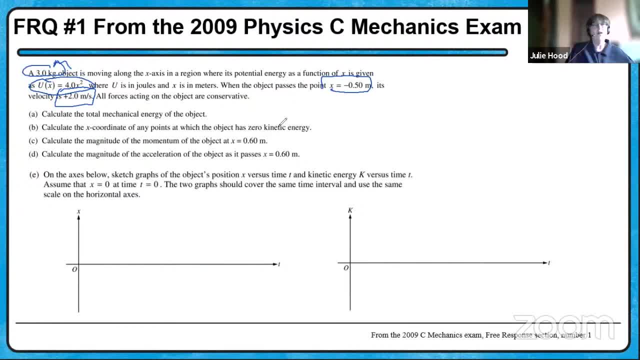 when the object has no kinetic energy at all. And then What's nice I like about this problem is they have you find the momentum and the acceleration at x equals 0.6 meters, And then you've got to sketch the displacement time of the particle and also the object's kinetic energy. 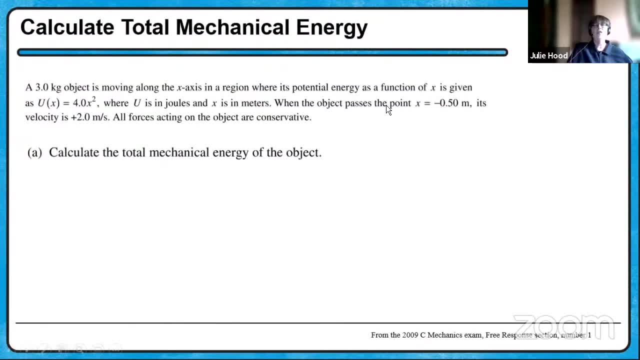 So let's do that. First things first, let's find the total energy in the system. Well, this is our function. Remember, the total energy is going to be whatever the potential is plus the kinetic at this position. So let's see what it is. 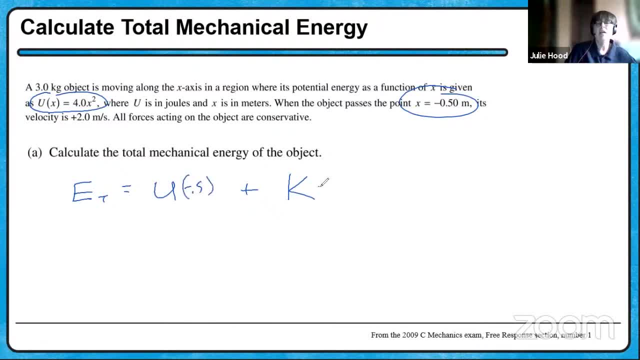 At negative 0.5 and negative 0.5.. All right, So they tell us what the velocity is. That's great help. The potential we actually have. We have to plug it in into our function And when we do that, 4 minus 0.5 squared, we find that, oh, there's one. 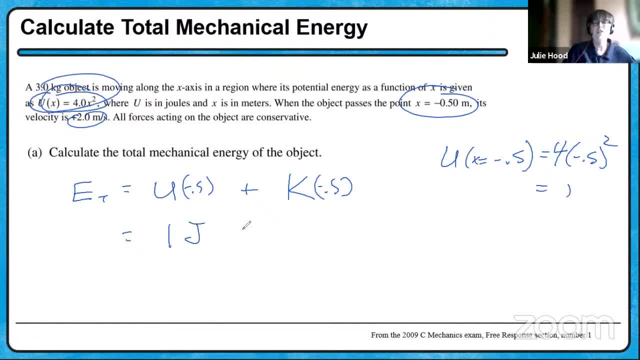 This equals one. There's one joule of potential energy And the kinetic energy is: hey, kinetic is 1 half mv squared right, So 1 half. The mass is right up there, 3 kilograms, And the velocity when the object is at this point is 2 meters per second. 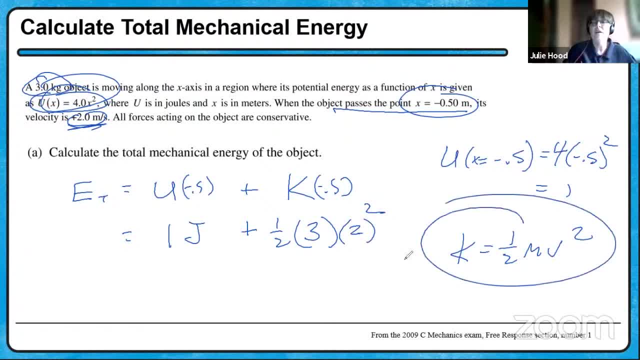 And we have to square that because that's how kinetic energy works. And when I square all of that, I get, let's see, 6.. So I've got 1 joule and 6 joules. I've got 7 joules of mechanical energy. 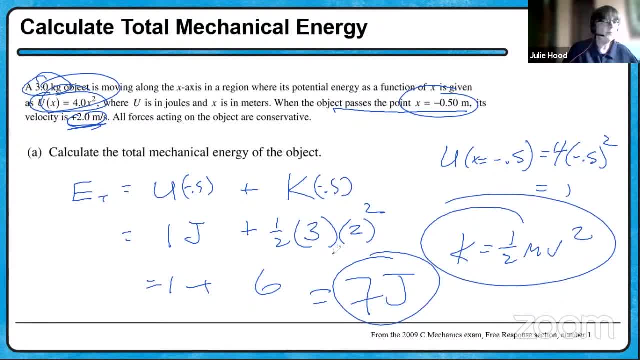 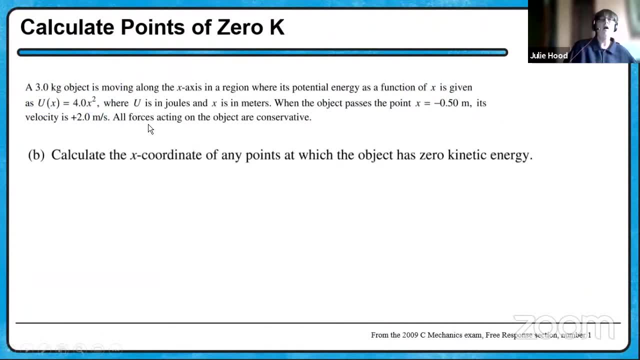 This object. It's always going to have this much energy. Good, Then let's just save that idea when we go on to the next part of the problem. Oh, now we have to find out where the object would have zero kinetic energy. 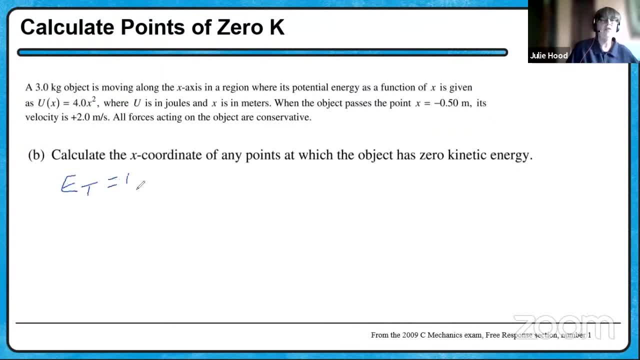 Well, we already know the total is U plus K And they're saying zero kinetic energy. So this part's zero. The total energy. we found that it was 7 joules And the potential is. here's our potential function. 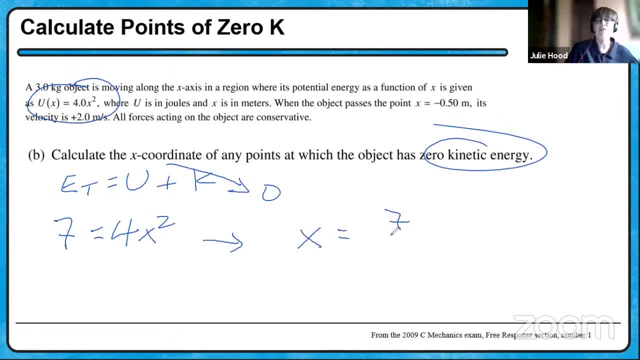 So all you have to do is solve for X, 7 over 4, take the square root And hello. don't forget there's a positive and a negative root, That if you forgot the negative sign, you didn't get all three points. 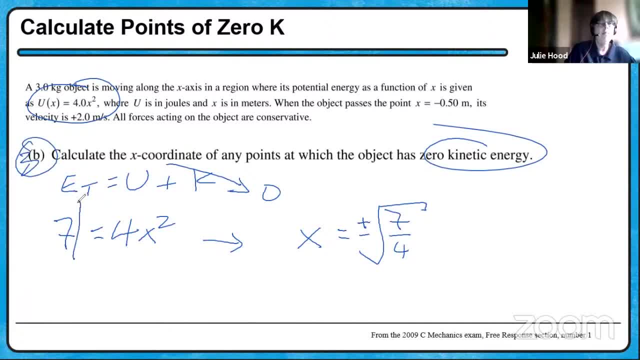 This was worth three points: One for making the substitution And one for making the substitution from part A. Even if you got the wrong total energy in part A, you lost that point. But if you used your total energy that you got in part A to do this problem, 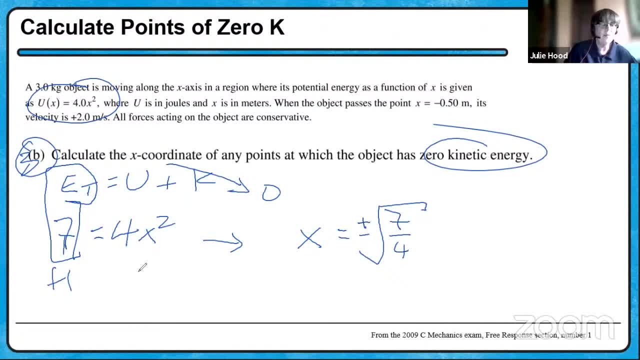 then you would have received credit, that point, for making that substitution. And then they wanted you to make this connection. of course That was worth a point. And then the third point was actually indicating both a plus and a minus. Now you could get your calculator out and say, oh, it's about equal to 1.3 meters. 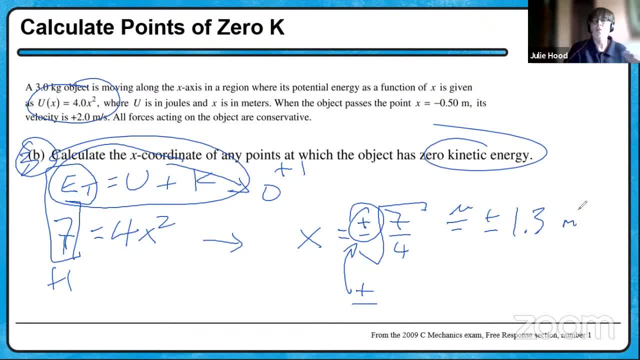 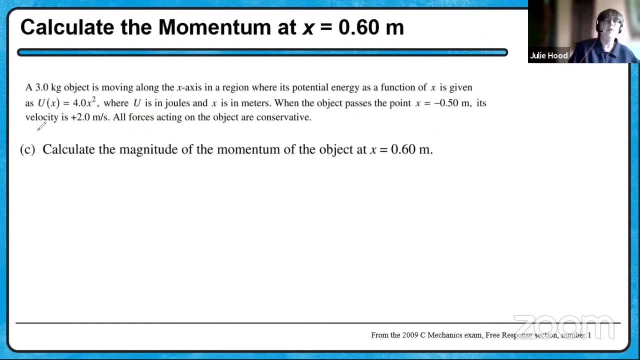 That's where the object will have no kinetic energy. All right, Let's go on and look at the next part. Oh, we want to find the momentum. OK, well, I know what momentum is. Momentum is mass times, velocity, And we're just looking for magnitude. so we don't care if it's positive or negative. 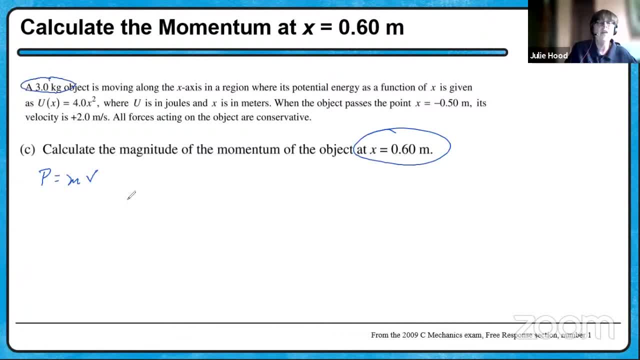 But we need to find. we know the mass, and that's not changing, But we need to find the velocity when the object is right. here, Remember, the total energy is the potential plus the kinetic, And that has to be 7 joules. 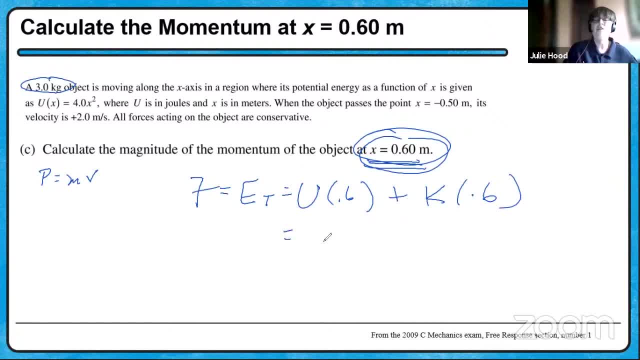 And you can do that. OK, All right, So you can figure out how much what your velocity will be, because the potential at 0.6 is going to be. here we go 4 times 0.6 squared. 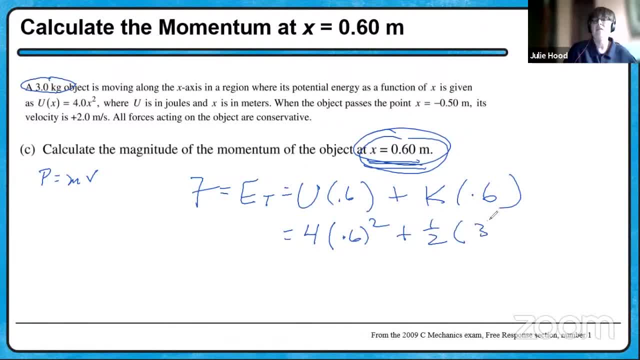 And kinetic is 1 half mass times velocity squared, And when you solve this for velocity, you're going to find that 1.93 meters per second is the velocity, The velocity at this location, And that's all, because energy is conserved. 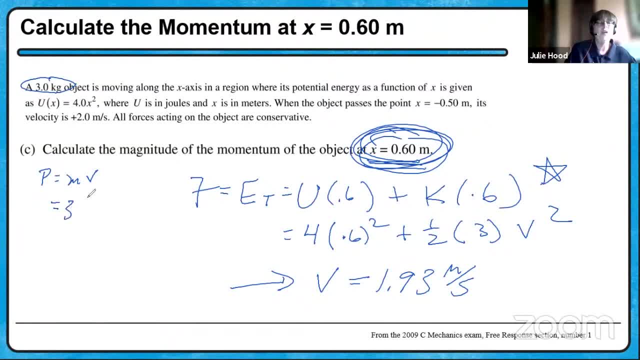 Love energy. We've got a mass of 3 kilos and a velocity of 1.93 meters per second, So we have a total momentum of about 5.8.. Don't forget your units: Kilograms- meters per second. 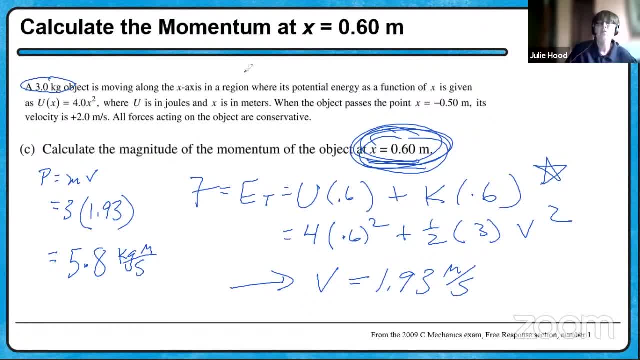 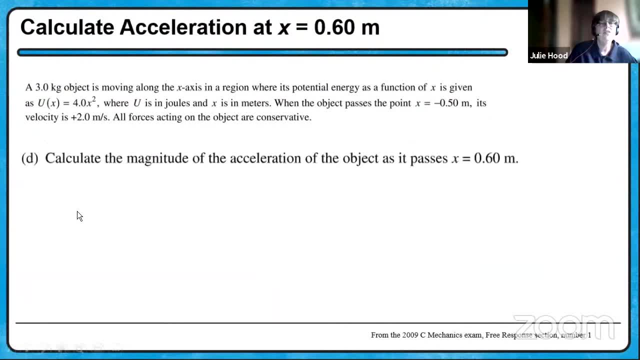 That's the units of momentum. Excellent, That's worth three points. Lots of energy conservation. Are you seeing that? It is just a really big deal. Now we want to find the acceleration. Hey, remember this equation: F equals ma. 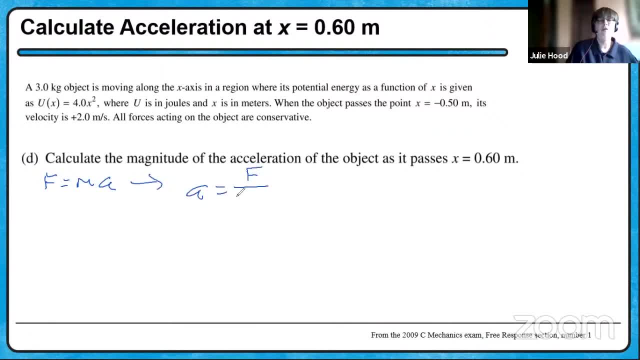 Oh, I know you do So. a is f over m. How do I get f? Oh yeah, F is minus the derivative of the potential function at this location. Well, let's just find the derivative. Let's just find the derivative of this function. 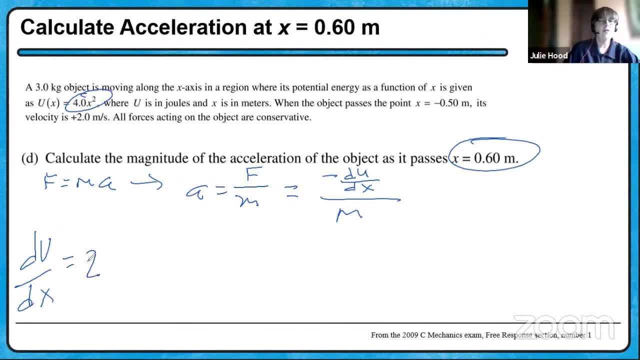 All right, That's going to be 2 brought down. Oh, that's an 8.. And reduce the exponent by 1.. Oh yeah, I remember how to do calculus, So we've got minus. Don't forget the minus sign. 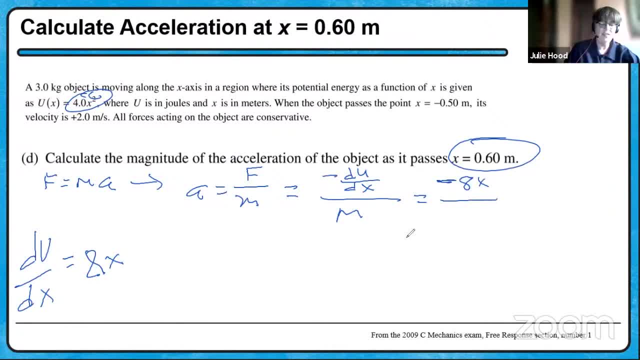 8x over the mass And the mass is the mass All right, The location All right. The acceleration is 0.6.. And the mass is- oh good, I remember It's 3 kilograms. So our acceleration is well they're. 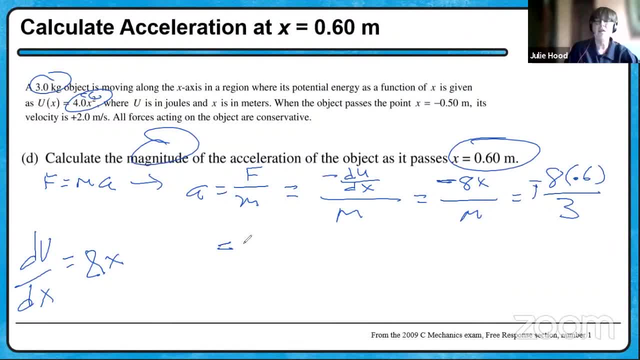 asking us for the magnitude, So don't worry about the sign there, But the magnitude ends up being about 1.6 meters per second squared. Now here's a really cool thing. We're going on with this problem. We're going to do some graphs. 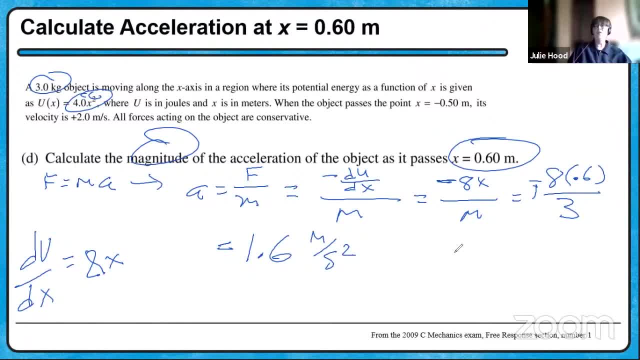 And I want you to notice something. I want you to notice that the force equals, of course, ma, But it also equals minus 8x. And mass, of course, has a numerical value, But what I'm seeing is acceleration is proportional to displacement. 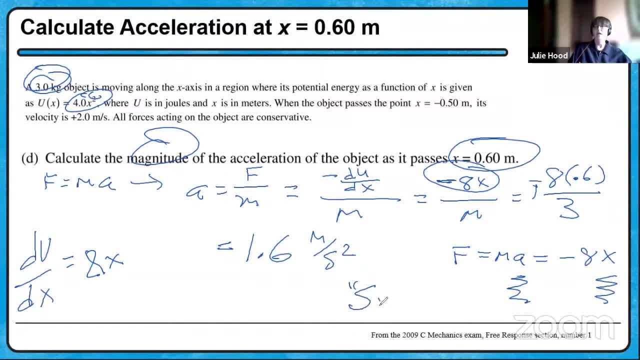 And that should ring a bell. OK, All right, All right, All right. Simple harmonic motion. This is going to help us do part e, So let's look at part e, Part e. remember the last part of this problem. 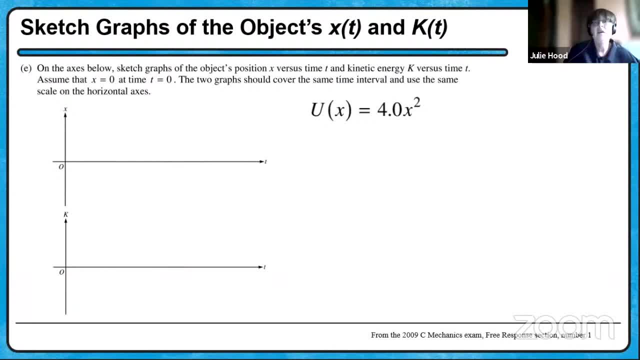 They want us to sketch the displacement time graph, And then they want us to also sketch the kinetic energy versus time. When I studied simple harmonic motion, they didn't write down the kinetic energy, They just got a video of this. So let's see what happens. 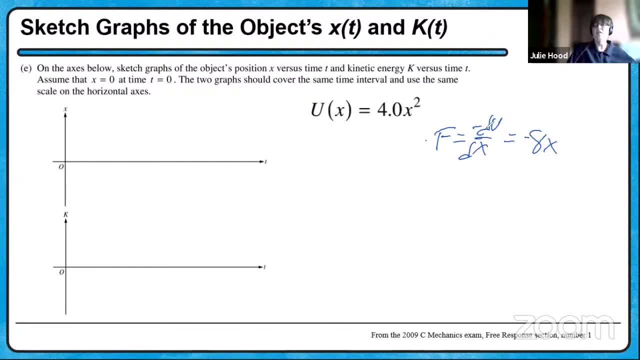 So what we're going to do is we're going to get the drag of the mass, of the mass, And what we'll get is that we get the drag of the mass And we get a little bit of a problem, And we're going to look at the integral of this. 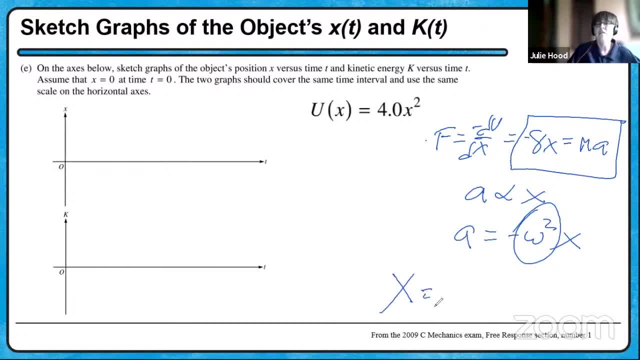 All right. So if this is equal to ma, then that's going to change. the solution to that is some amplitude cosine omega t or sine omega t, depending on your initial conditions. So we've got sinusoidal motion, but we need to look at the initial conditions, or 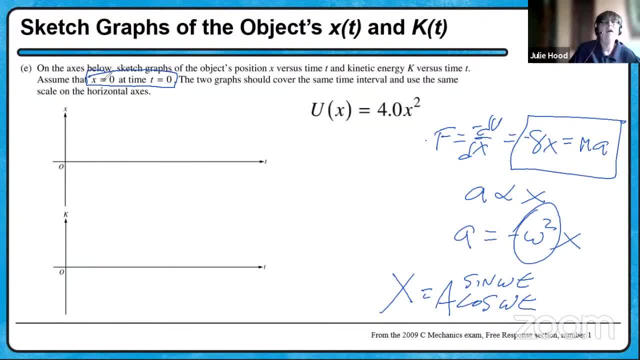 we won't. we'll lose a point if we just sketch in a cosine At: x equals zero, time equals zero. So what we have going on is a nice sinusoid. Hey, this is an entire period of oscillation, And if 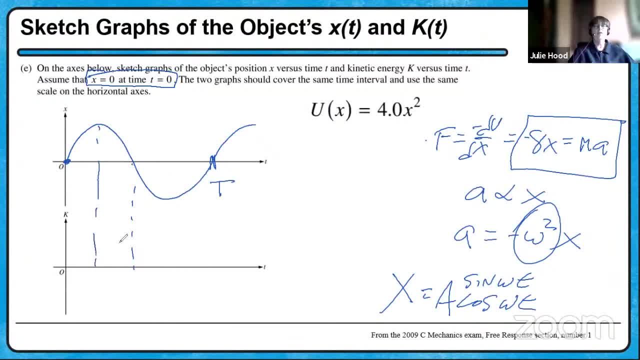 I were you, I would bring these down so we can align them. Let's remember that k is one half the kinetic energy, one half m v squared. If I know x, well, x in this case is some amplitude. So if I know x, well, x in this case is some amplitude. So if I know x, well, x in this. 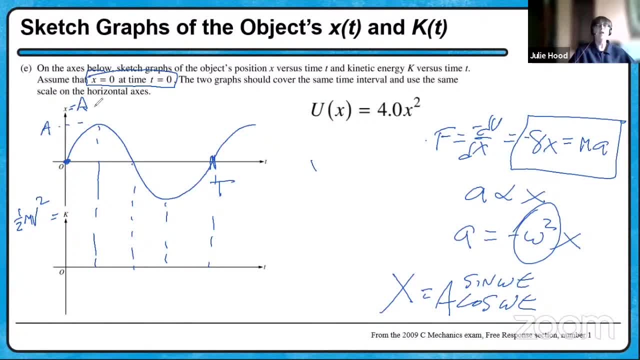 is some amplitude. So if I know x, well, x in this case is some amplitude. So if I know x, well, x in this is some amplitude. I don't know what that amplitude is today, but sine omega t, The velocity. 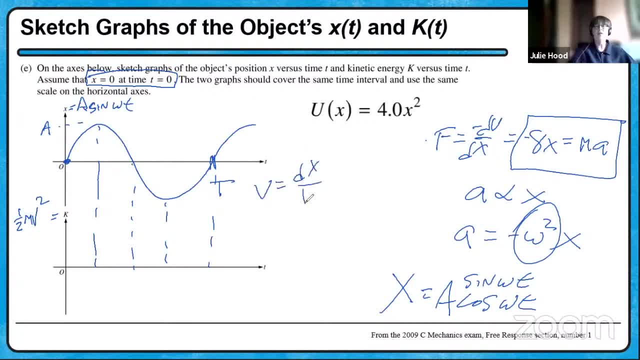 that I need to find is going to be the derivative of x. So what's the derivative of the sine, The cosine? Pull the omega out. Now be careful, Don't just sketch a cosine, because it's velocity squared. You're going to have a maximum velocity when you're at a minimum of displacement. So I would go ahead. 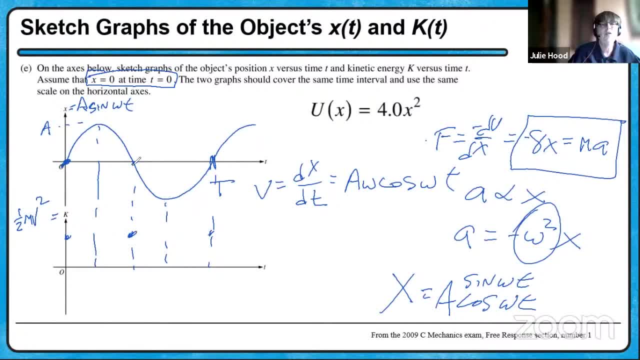 and sketch those bits in first, And when you've got maximum displacement you've got no velocity. So this is our. it's not really a nice, it's a little more smooth, but that's our kinetic energy Kind of cool. 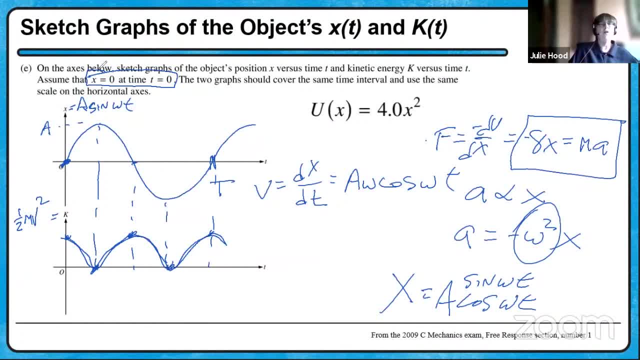 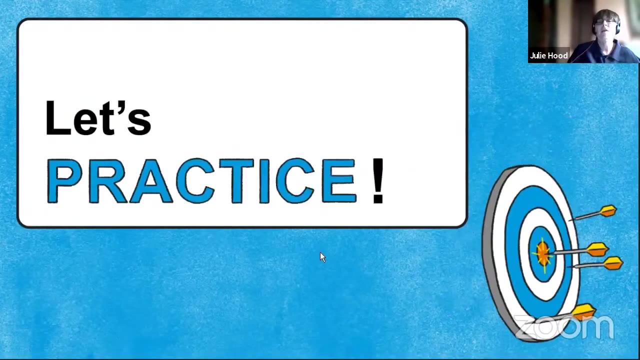 And yeah, they wanted you to use your initial conditions so that you had a sinusoid, They wanted you to plot for at least one period of oscillation And they wanted you to match up the minima and maxima to get full credit on this Great problem. Remember this was from the 09 exam, But I want to. 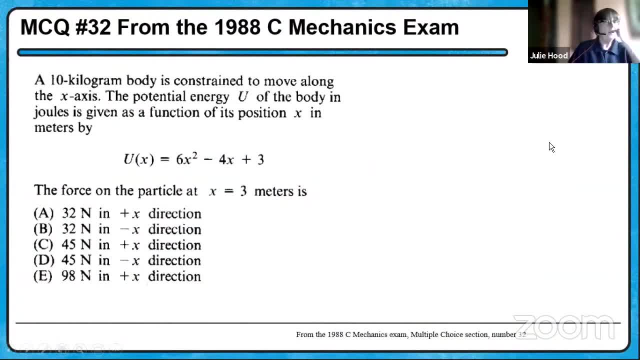 show you some multiple choice problems, And this one came from 19. 88. Great problem. They give you the potential energy And they want you to find the force on the particle. And guess what we're going to use? Oh yeah, We've used this a few times today, haven't we? 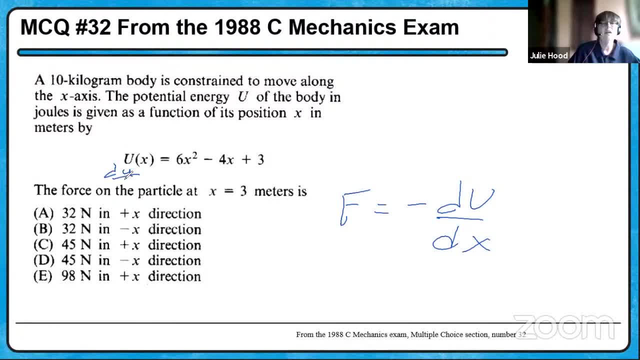 So let's just take the derivative of this guy. Easy peasy, Bring the 2 down Minus 4.. That is a constant And we're talking about At x equals 3.. So at x equals 3, then we've got 12 times 3 minus 4.. 12 times 3 is 36 minus 4 is 32.. 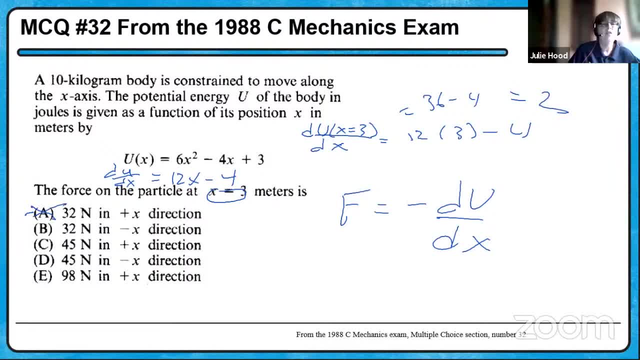 Be careful, Be very careful. This is not the right answer. These certainly can't be the right answer. But don't forget the negative sign. So 32 newtons. You betcha? This should have said 32.. But in the negative x direction. So B, B is your answer. 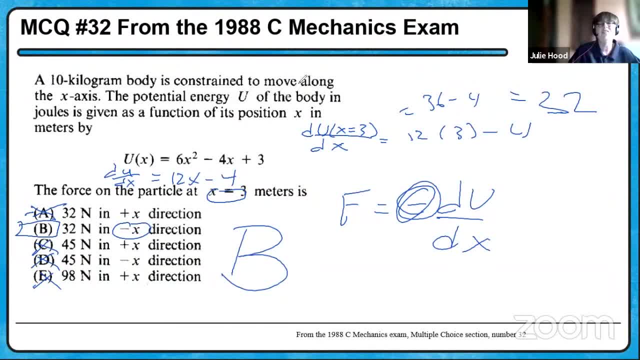 They're always going to put answers down that seem so right And unfortunately you make a little mistake And you think, oh, I got it right, because the answer was there. No, That's called a distractor. Be very careful, Take enough time. 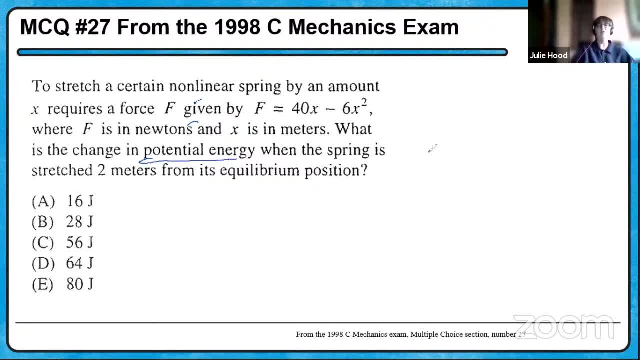 Now here we're, given the force And we want to find the potential energy. Look, if the force is minus du dx, then guess what u is? Well, let's just do something they don't like us doing in math, but it works. 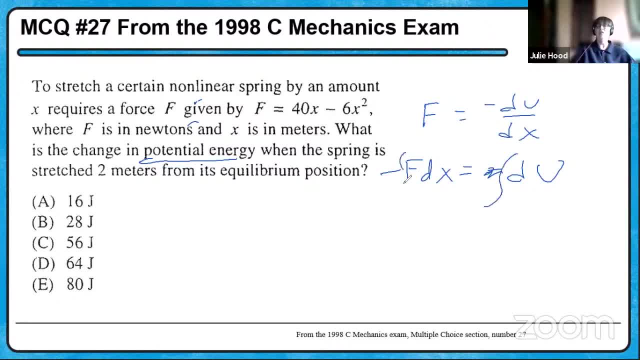 So I do it. Bring the negative sign over and take the integral of both sides. Oh? u is just going to be the negative integral of f? dx. I know how to integrate 40x minus 6x. squared You ready for it? 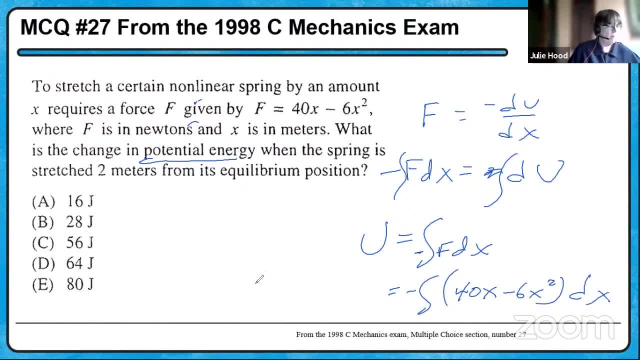 Well, it's going to be a function whose derivative is this: integrand, And that would be minus 20x squared plus 2x cubed. Fine, Now we plug in when x is 2 meters and we get minus 22 squared plus 22 cubed. 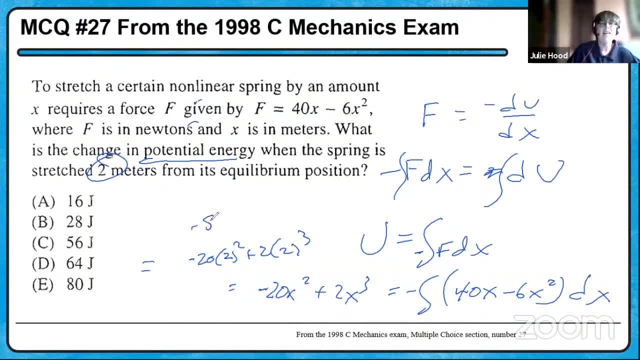 And that equals, oh, minus 80 plus 16 or minus 64. And I do a quick scan and, oh my gosh, I don't see any negatives. Yeah, we're just talking about a change in potential energy. 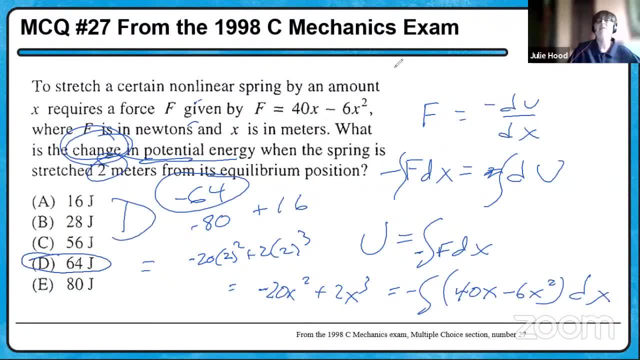 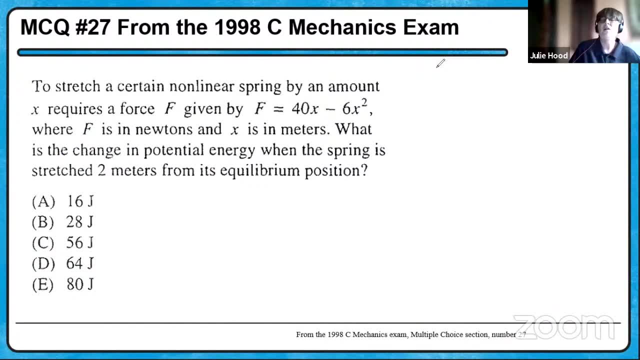 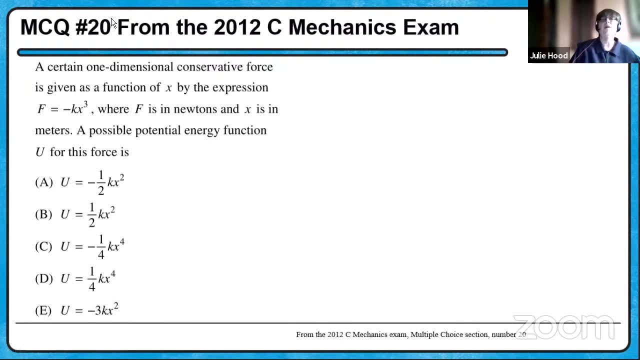 So here's your answer d Again, these sessions are recorded and housed on the AP or College Board AP YouTube channel, So you can go back and look at these and take a little more time than I may be taking, Or you could go back and watch me in double time. 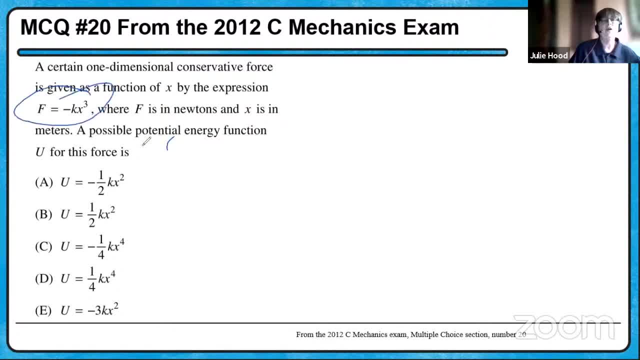 Blah, blah, blah, Mickey Mouse. Okay, so we've got a force. We want to find the potential energy. Just take the derivative. No better yet we want to find the potential energy. Take the integral of the force. 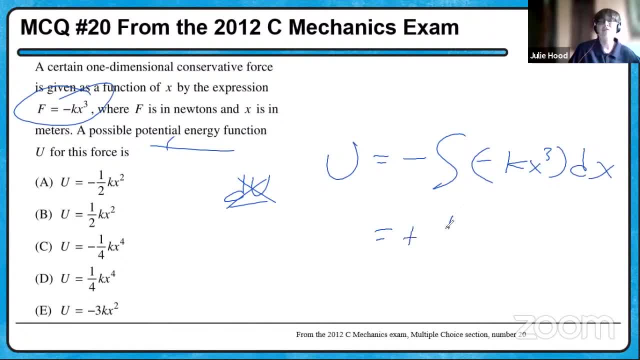 Now those negatives are going away, But we've got one-fourth kx to the fourth. Remember the integral is a function whose derivative is the integrand Fundamental theorem of calculus. That much I do remember. So d is your answer. 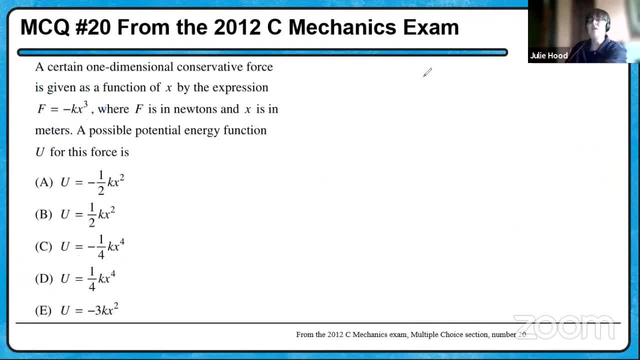 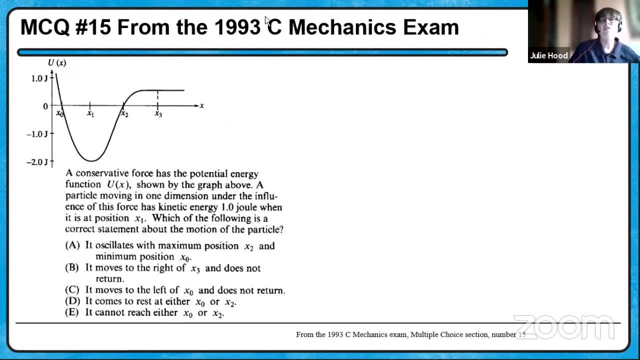 And I think I've got one more for you. So that's good, We're doing just fine with the time. I've got actually two more. Even better, I've got this one. I've got a conservative force. Okay, so there's the potential energy. 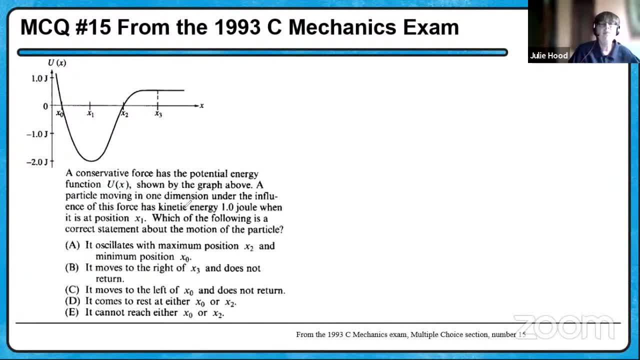 Conservative force, Energy is conserved. They're telling me that this object has one joule of kinetic energy when it is at position x1. Now the total energy is u plus k And at x1. u has minus two joules. 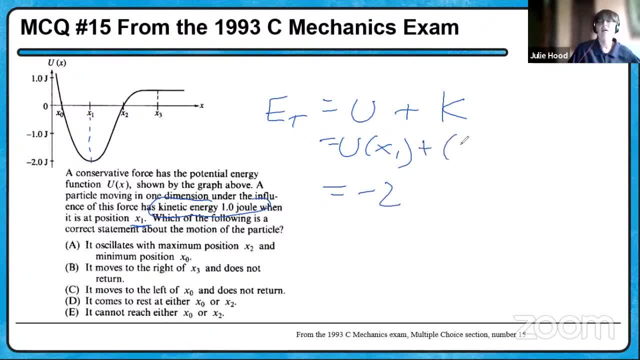 And they're telling me that at that position, whoops, k, whoop of x1 has there it is one joule. So here's how much total energy this particular particle has. It's okay, It's got a negative energy. 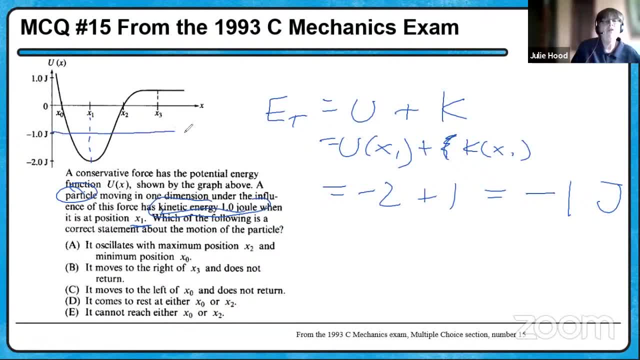 So I go ahead and I draw, I draw my horizontal line And I know that my particle can't get to the left of here And it can't get to the right of here. It won't have enough energy. That particle can only oscillate between these endpoints. 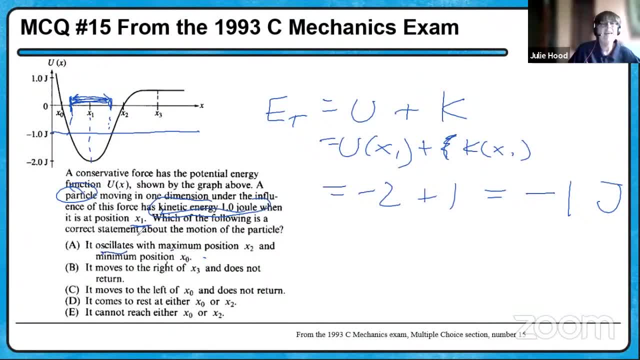 So it can't. Certainly it oscillates, but it cannot get to x sub zero or x sub two. So a is not an answer. It certainly can't move way over to the right of x3. It can't even. It can't even get to x3.. 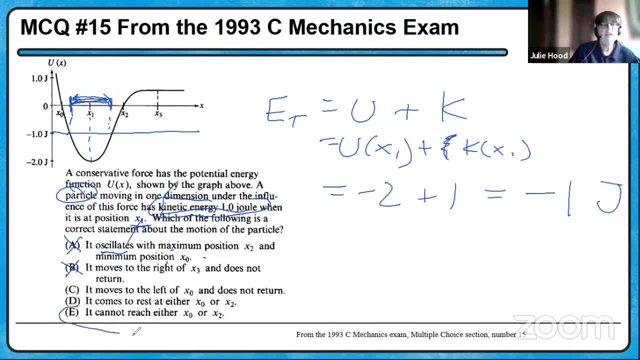 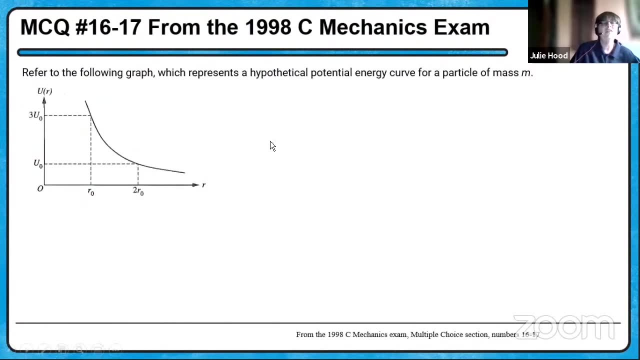 And on and on. you know, basically e It can't reach x0 or x2.. Can't get there Too bad. So e is your answer And there's another one here from the 98 exam And we had this nice potential energy graph. 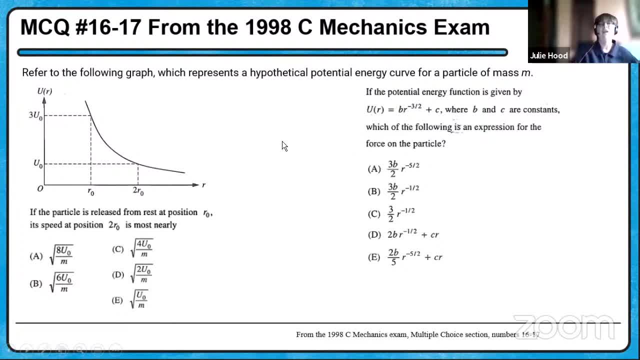 And what I liked about this is it actually had two parts. And again, energy is conserved- And I'll let you try this on your own, But with energy being conserved. remember change in potential, change in kinetic equals zero. 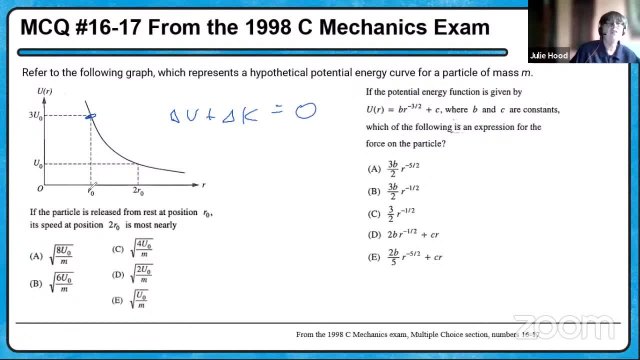 So they're telling me that the objects at rest at r0. So that means the total energy in the system is 3 u0. And it's at rest. So let's see. So when we go over here to this position, they want to know how much speed we have. 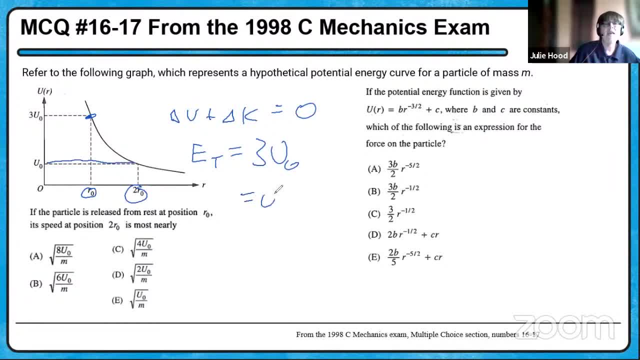 Well, I have this much energy tied up in potential And the difference is going to be the kinetic energy. So fine, Do a little math. I've got 2? u and another 2 brought up. Divide by the math, Take the square root. 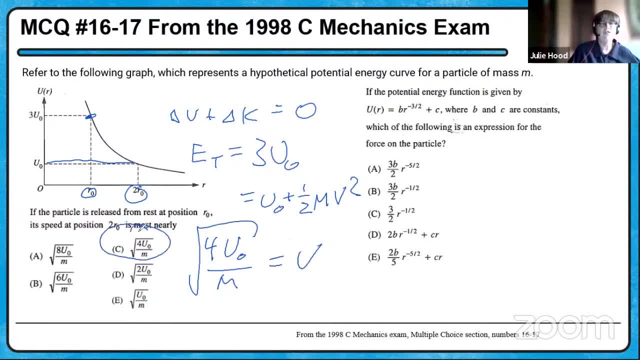 And that's my velocity. I hope that's one of my choices, It sure is. And then this guy: I've got my potential energy And I want to find my force. Just take the negative derivative And you'll find that there's your force. 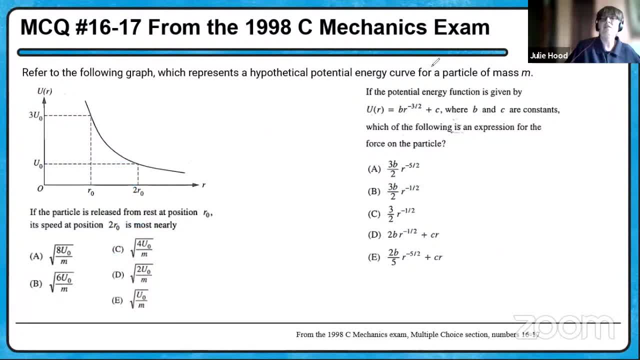 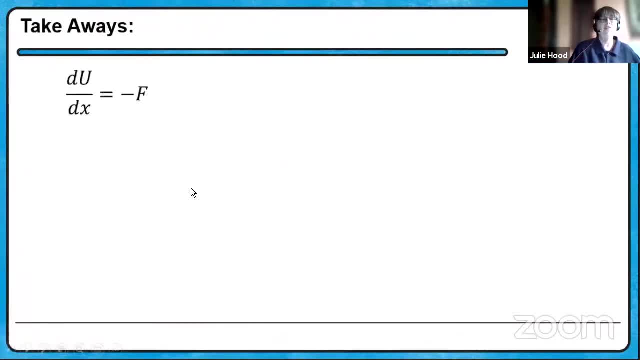 All right, I think we covered a lot of topics today, And what we really need to take away from this review is this equation And the fact that you could also look at this equation in the form of getting the potential energy by taking the negative integral of the force with respect to displacement. 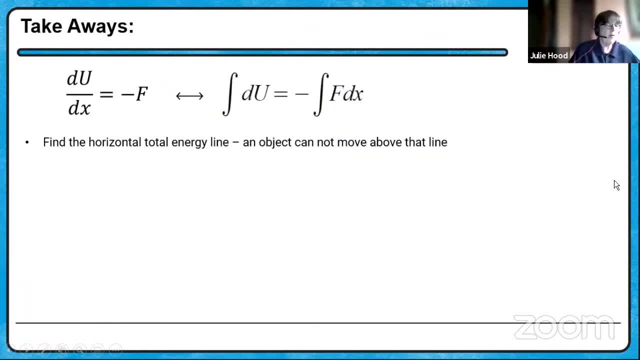 Find that horizontal total energy line. Remember, I did a free response problem, the one from 1987, where we definitely looked at the horizontal total energy line. I also used the total energy line when we looked at that multivariate, And I also did a free response problem, the one from 1993.. 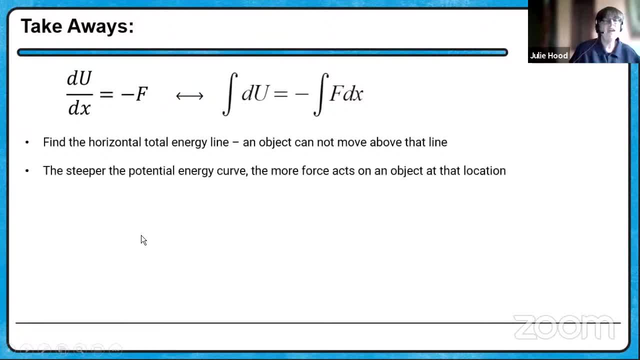 And I also used the total energy line when we looked at that multivariate. And I also used the total energy line when we looked at that multivariate And I also used the total energy line when we looked at that multivariate. Other takeaways are the steeper, the potential energy curve. it just means there's more force acting on the object at that location. 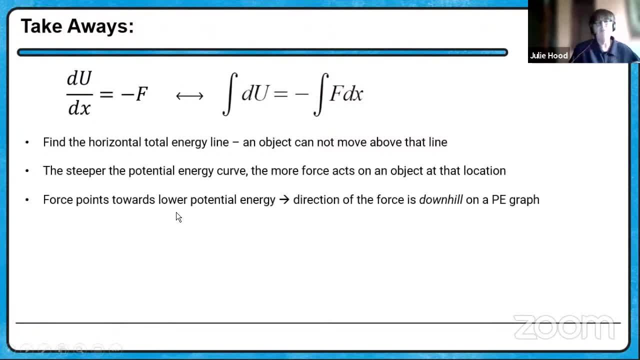 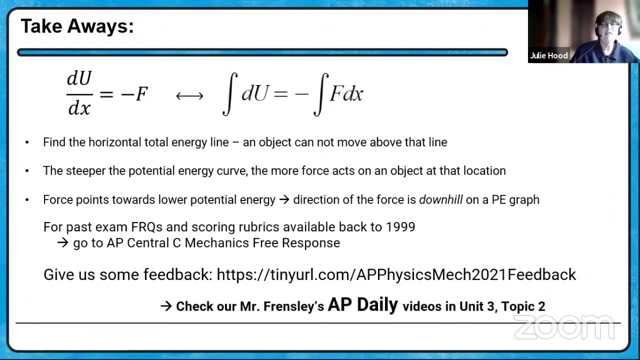 Force always points to bring an object to its lower potential. Go back to AP Central and find old free response And give me some feedback. I'd love that And definitely check out AP Daily videos, in particular Mr Frensley's from Unit 3, Topic 2, all about potential energy. 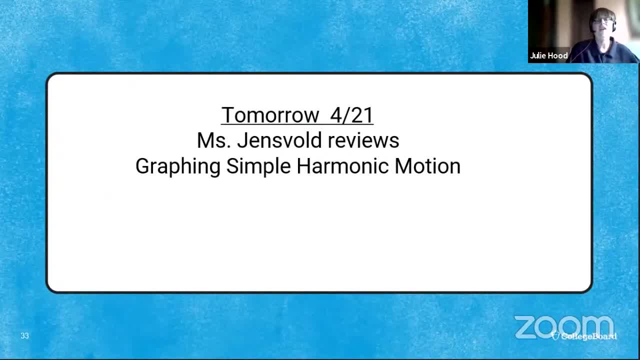 Tomorrow, come on back, Ms Jensfold will be here and she's going to review graphing simple harmonic motion. We talked about that a little today. She'll talk about it a lot more And on Thursday. On Thursday, I'm back with non-linear springs. 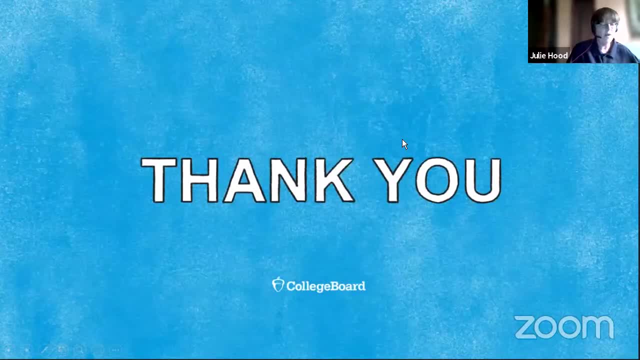 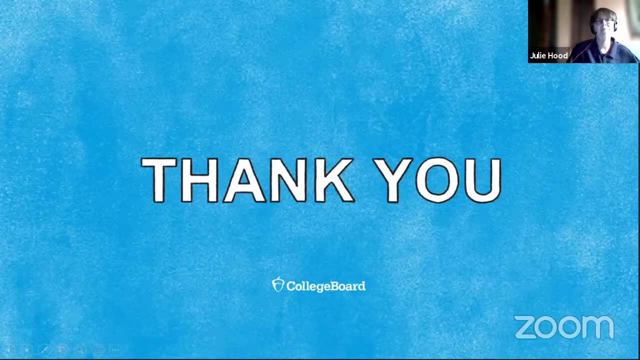 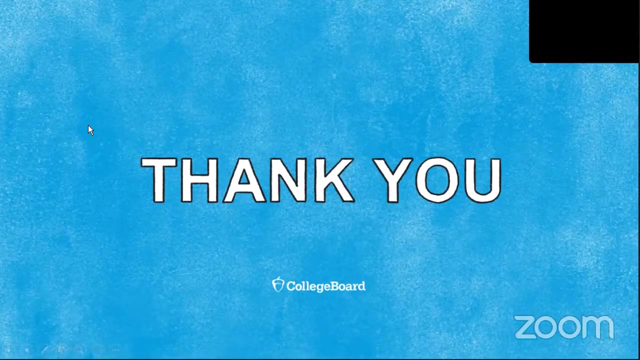 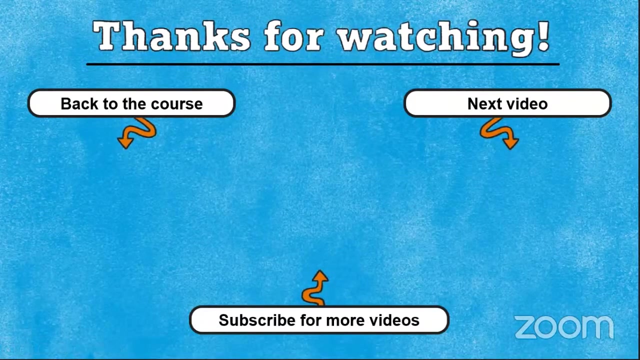